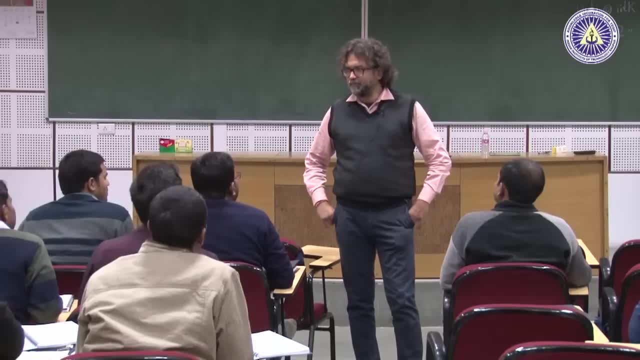 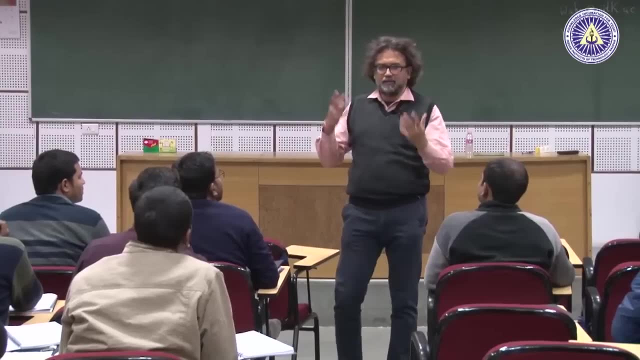 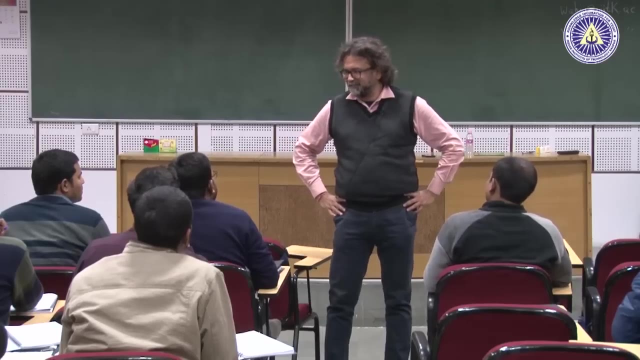 was one more batch which came before this and this is the second batch. ok, yeah, So I think we have. I have only half an hour actually, So I do not know. I mean, we I tried telling the last batch some things and I will try to sort of experiment with you also. I am. 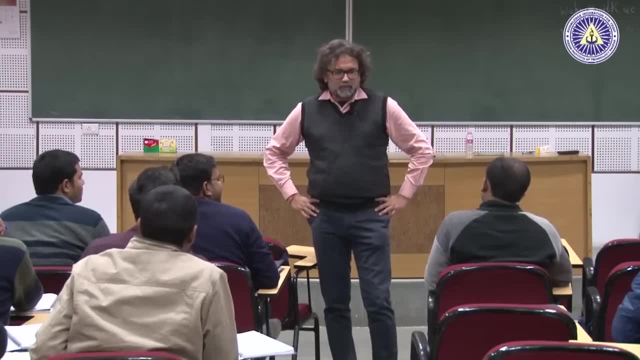 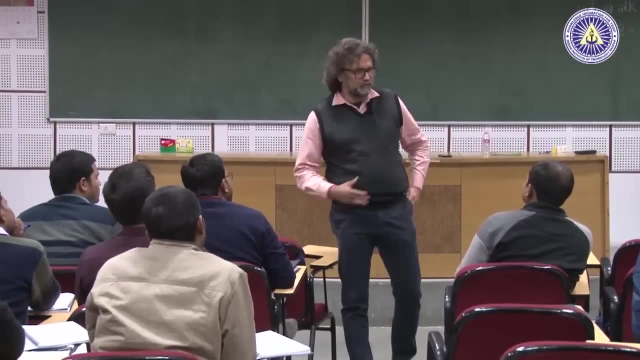 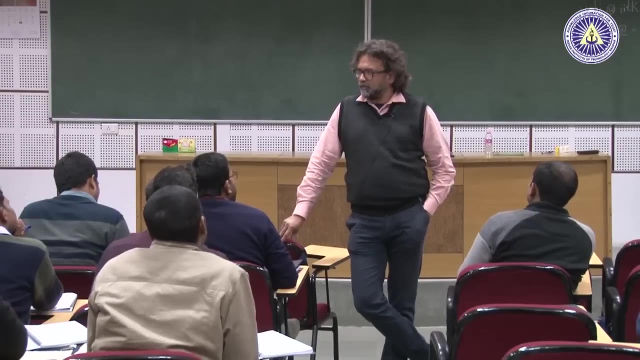 an experimentalist, Anyway. so it is basically to talk about teaching in thermodynamics and heat transfer. ok, and that is what I also teach. We have a core thermodynamics course which is done by almost all the across the institute, and we also have 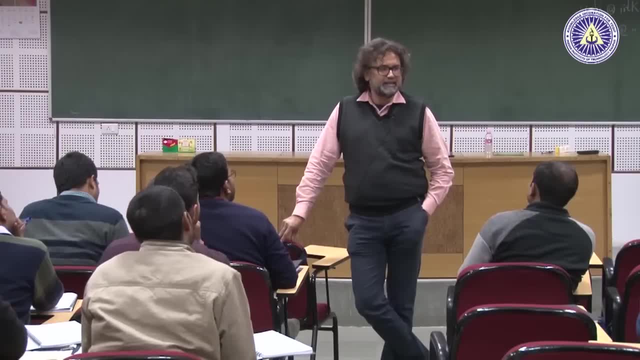 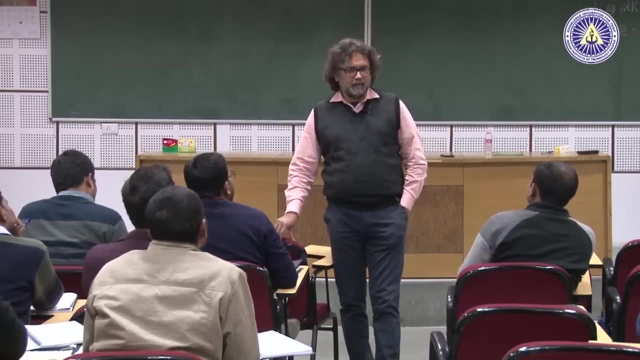 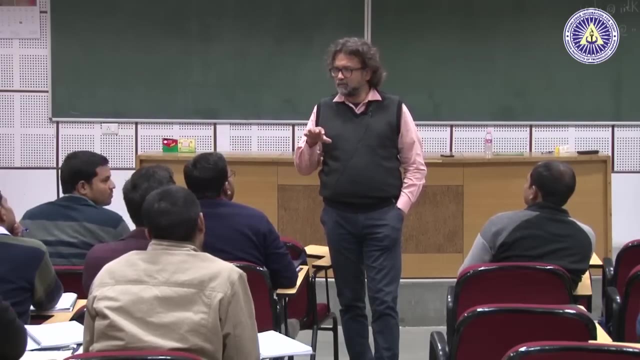 a heat transfer course, heat and mass transfer, which is done by the mechanical engineering students. It is a compulsory course in the sixth semester, ok, or the present semester I am teaching, in fact, And how many of you are trained in thermal or fluids? One, ok. 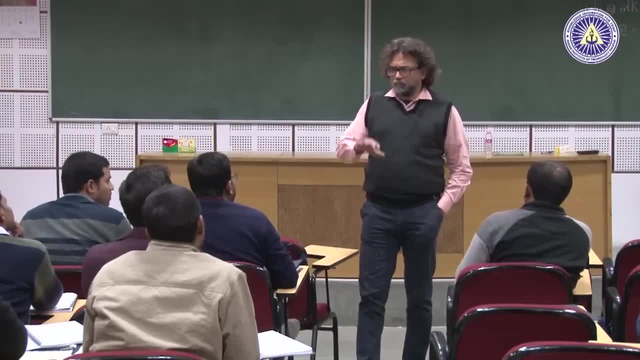 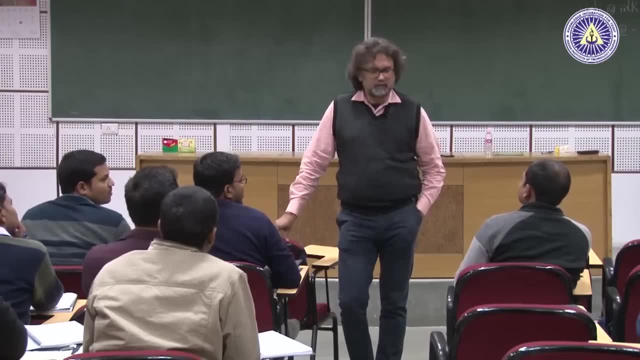 two, three. ok, Most of you are MTechs or PhDs also. No, most of you are MTechs. Sir, I have submitted my thesis. Oh, you have submitted your PhD thesis. ok, So, more or less ok, So anyway. so what I wanted to tell you was: 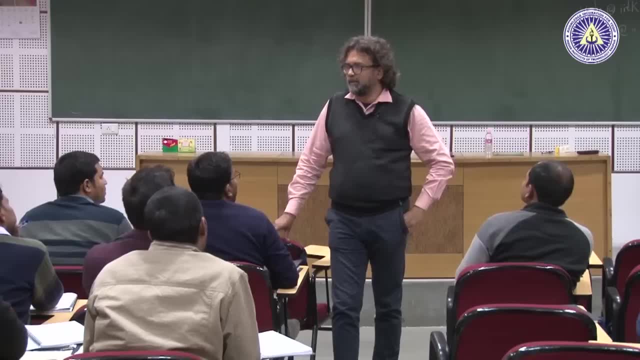 that Yes. So what I wanted to tell you was that. So, anyway. so what I wanted to tell you was that, look, thermodynamics is a vast course, So I do not know whether you will be you will. 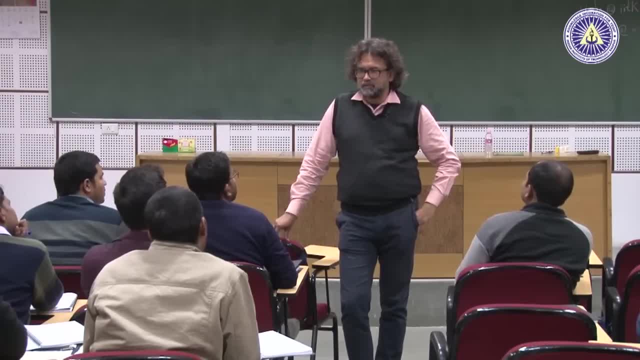 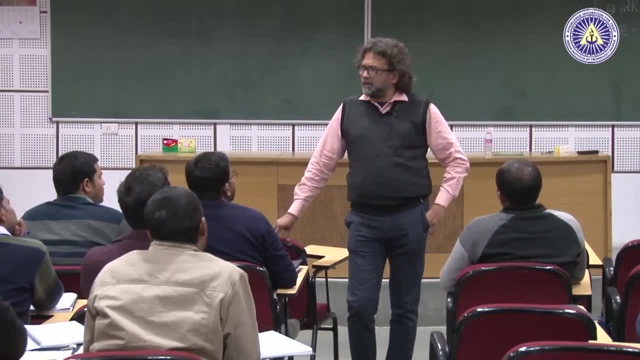 get a chance to teach or not? Heat transfer: of course many of you may teach ok, depending on your interest also and the type of institute which you are in, And there are plenty of books which are available in there. both of them are classical subjects, so to say ok. 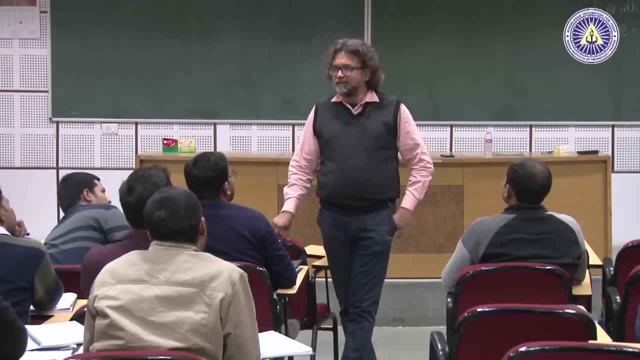 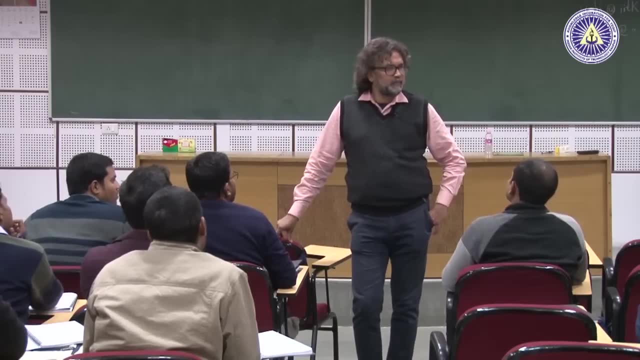 So plenty of books are available. Some of the books are user friendly, some are more matured, some are for more matured students or matured teachers, for example. Some of them are very user friendly And you know I have done a lot of research in the field. 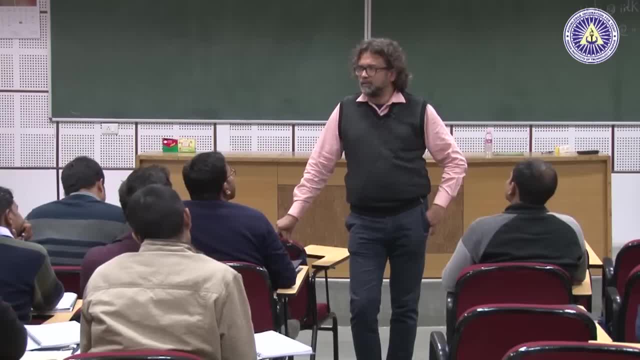 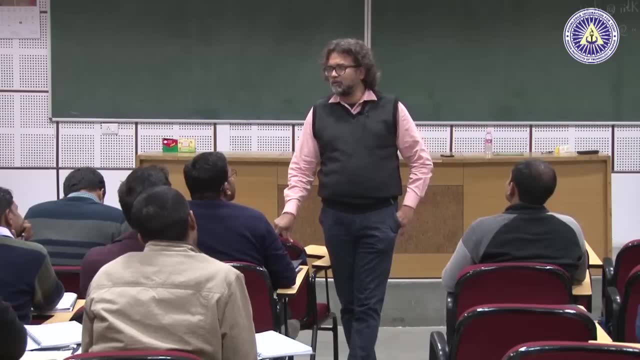 and right now one of the most popular books which we are using here in IIT also is the thermodynamics as well as heat transfer- is by a professor called Yunus Schengel. ok, So Schengel's book is pretty good If you really devote your time reading it- and try to Now. 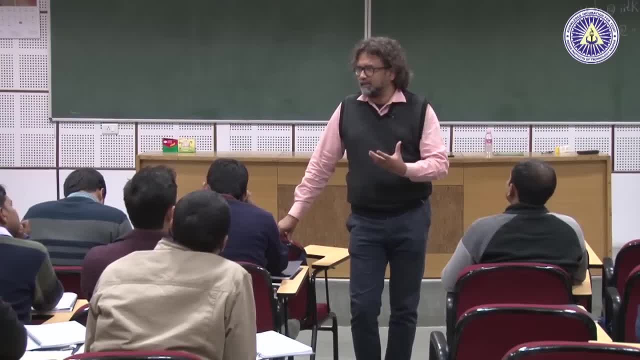 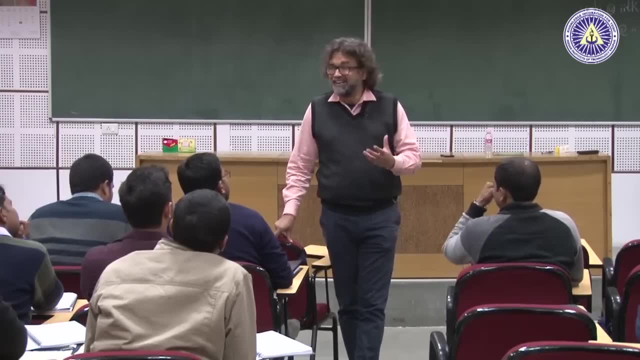 why that book is good and why I also like it as a teacher. I can tell you that two things. One is the book is very friendly. It talks to the students. I mean it talks to the reader. ok, There is a dialogue which 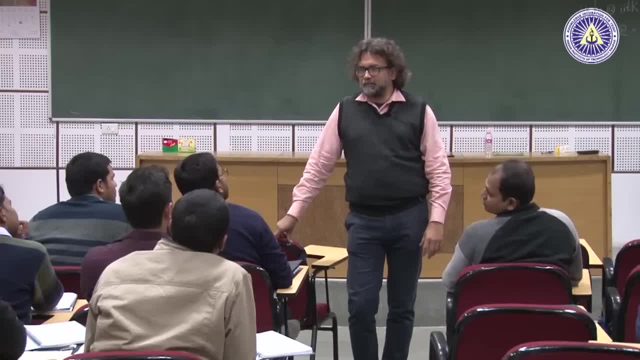 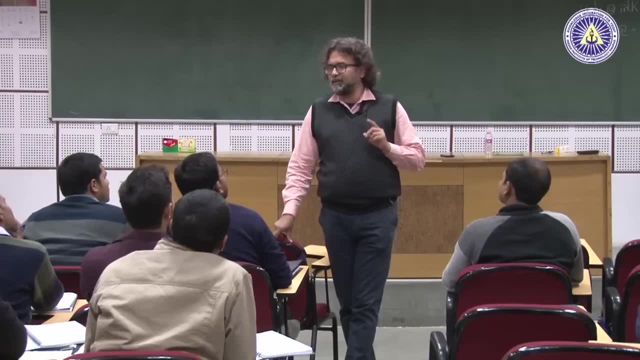 sets up, you know, between the author on. yeah, it is like a teacher itself. you know, it is like a speaking. The other thing which is more important, ok, is the fact that two things are important. One is that the examples which the book gives are very realistic, ok. 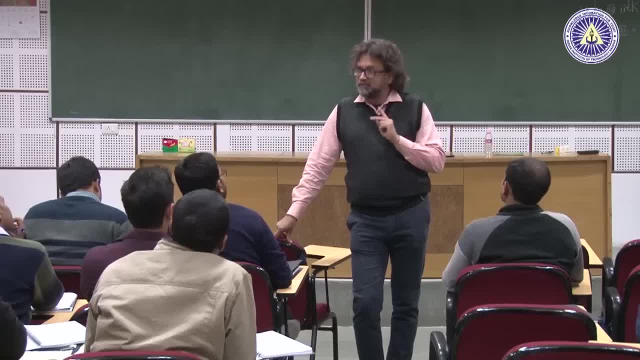 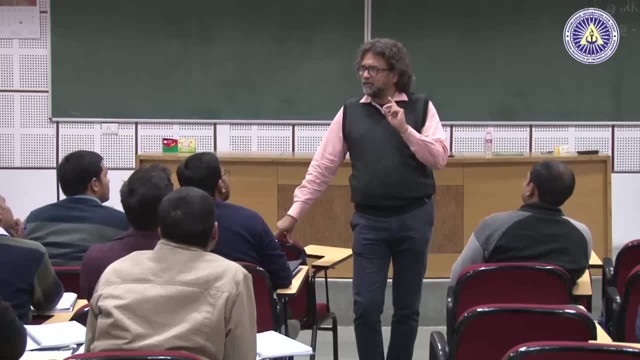 That means the data which has been taken, the assumptions which have been taken, the calculations which are done. ok, the calculations which are done are very, very realistic in what goes on in the industry, for example, or what goes on in the market, so to say. 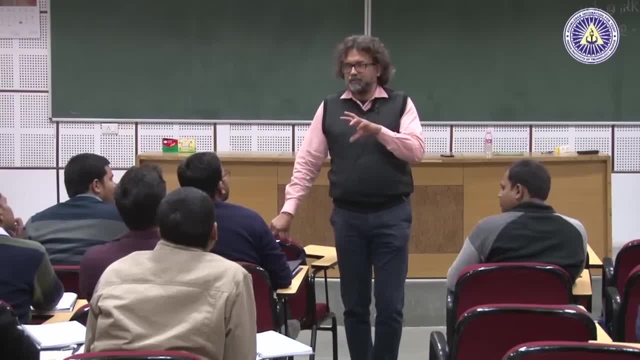 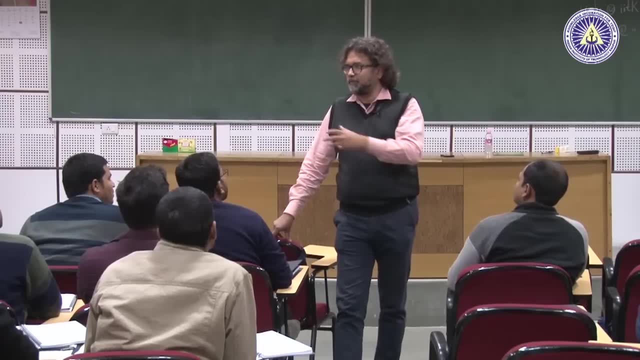 In our surroundings. Yes, in our surroundings. So that is one. The second thing is that it picks up- that word is important- surroundings. It picks up concepts from around you, isn't it? And then tries to put the theoretical framework and the you know, the theoretical framework. 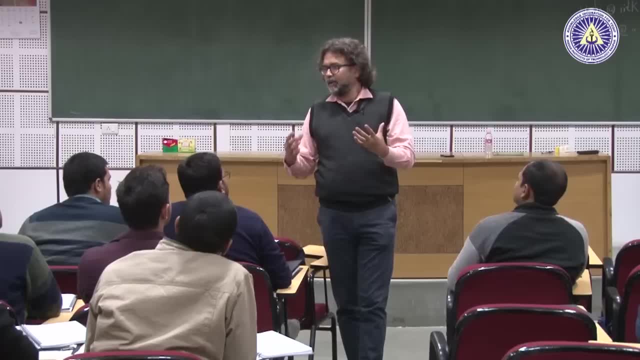 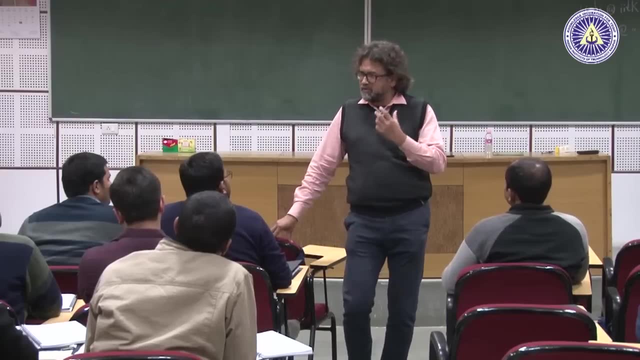 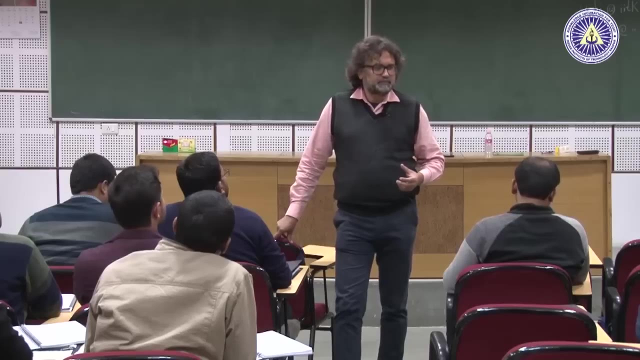 and give those examples and then connect the two. So I think it is very, very, very important as a teacher, ok, that you the subject which you are teaching, whether it is thermodynamics or heat transfer, or strength of materials or, for that matter, any other subject- you 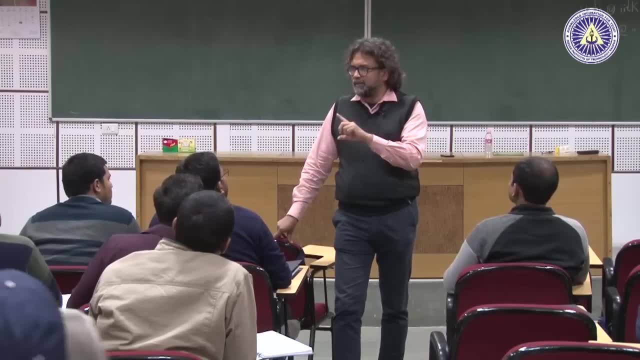 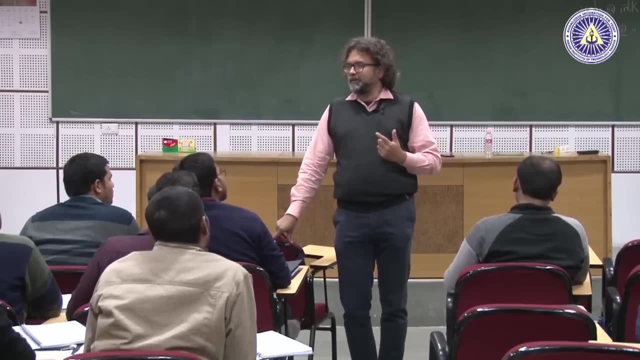 should be able to teach. you should be able in a way that the student connects to his environment. ok, The connect, the connectivity with the environment. that means the engineering. engineering is not in the book. Engineering came, then the books came, So we have to. 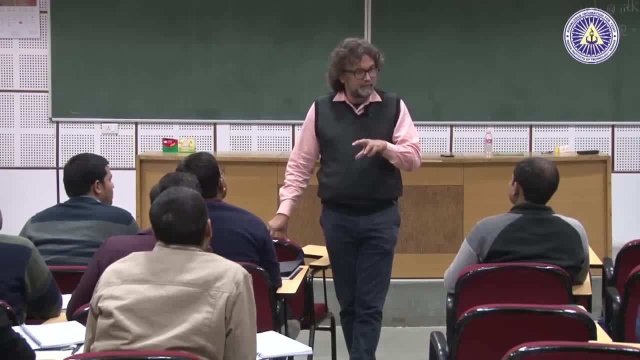 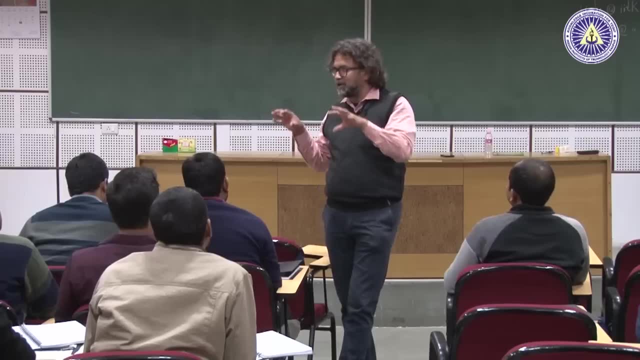 understand that the book is not where the knowledge lies. The knowledge is actually spread up everywhere. Book has formalized it. It has made your life easier. It has been segregated into chapters so that the delivery or the consumption becomes much more lucid. 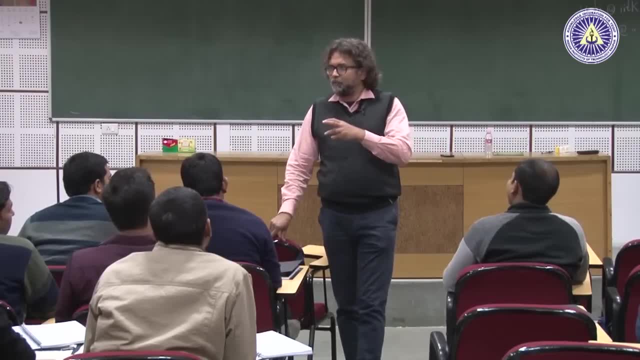 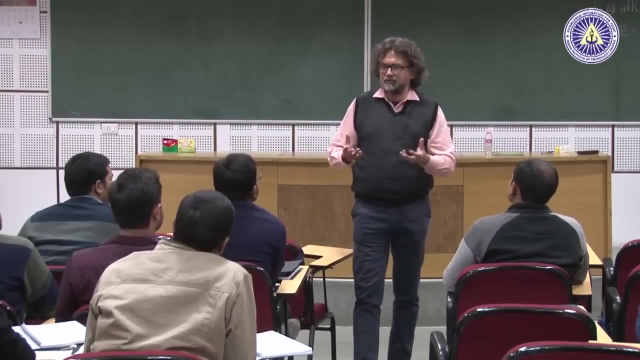 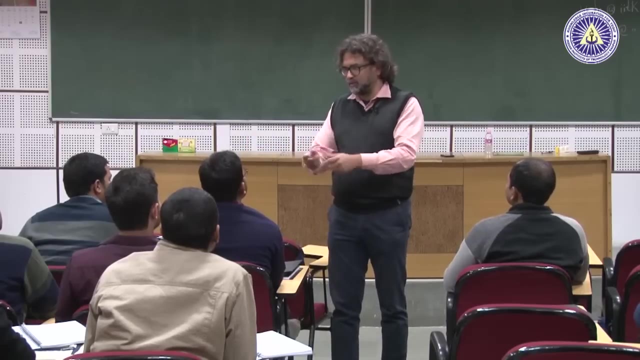 and interesting, for example. However, knowledge is around us, isn't it? That means, for example- I usually give this common example of, let's say, your finger gets burnt, you know. you are ironing the clothes in the hostel, ok. or your mother is cooking something and you. 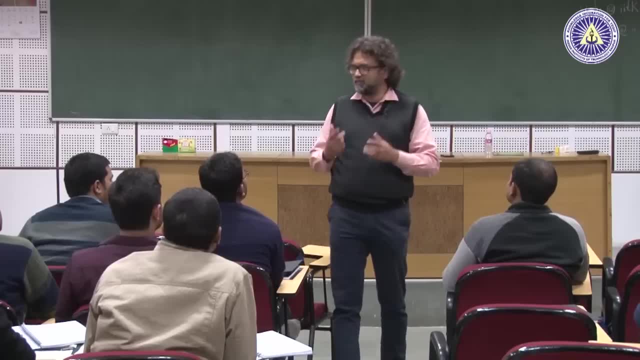 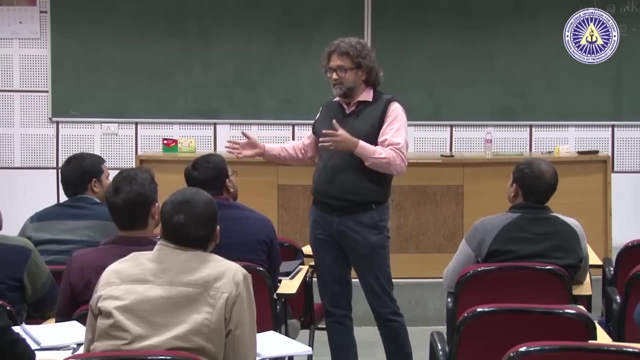 happen to touch- you know the hot tawa, for example, and the finger gets burnt. ok, Now one can. one can take this example of a finger getting burnt, and then all the equations of heat transfer, the energy conservation can be applied and you can teach them with that. 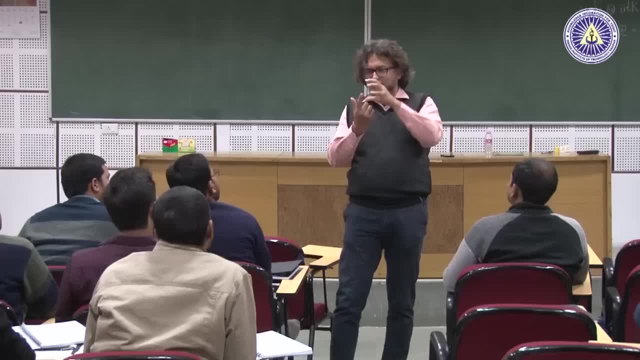 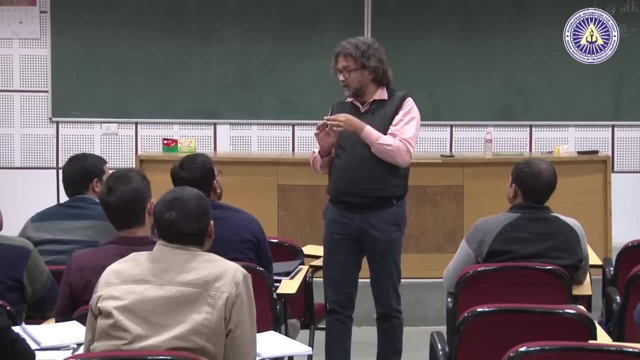 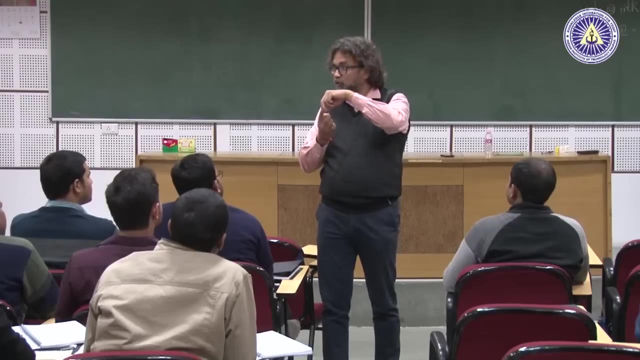 as an example, isn't it? Ok, You have. you have a mass of the object, You have some specific heat of the object, You have a thermal conductivity of the object- ok, Then a certain amount of energy has been supplied to the system, So you can make a control volume and the energy comes in. No, 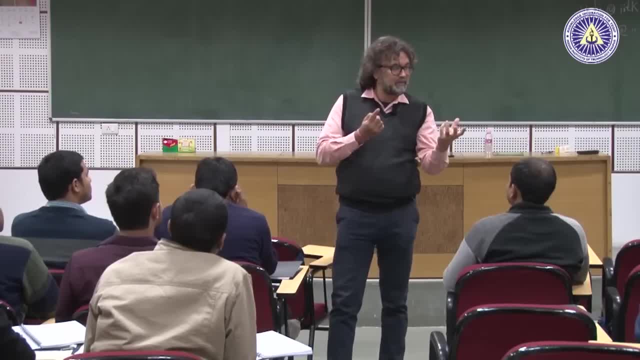 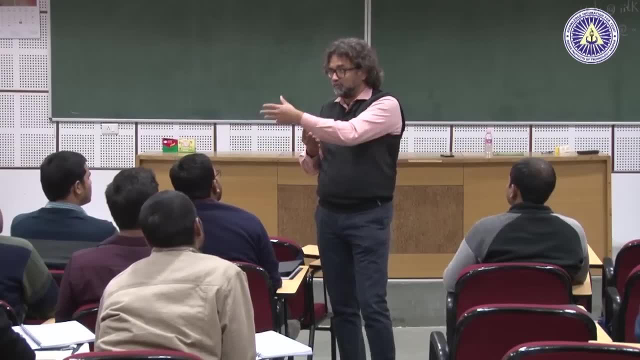 work is done. So that means the energy must be equivalent to the heat supplied, must go eventually to the internal energy of the system. So dq is equal to du plus dw. There is no dw, So dq must be equal to du. 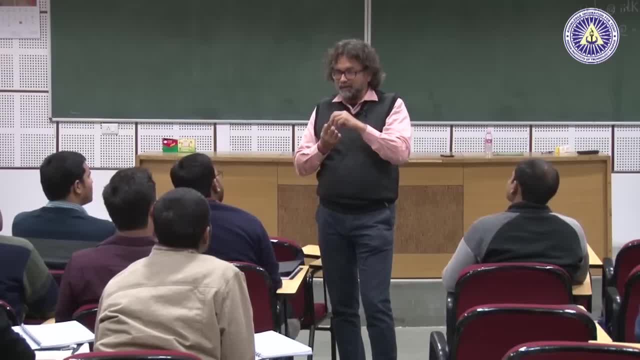 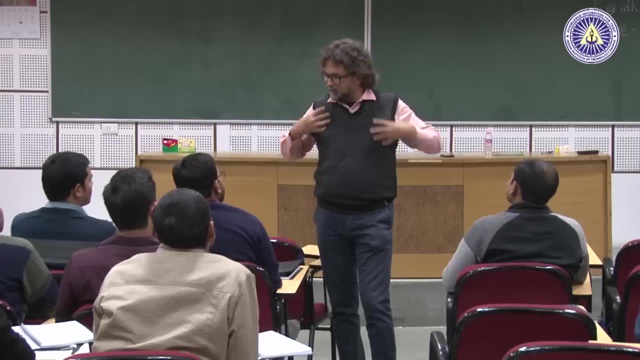 Isn't it? And then what does? what does that du do? Naturally, there is a rho and there is cp, and so that there is a delta t. So there is, it is a fixed temperature system, and there is a big body which is isothermal and a small portion has been burnt. So you 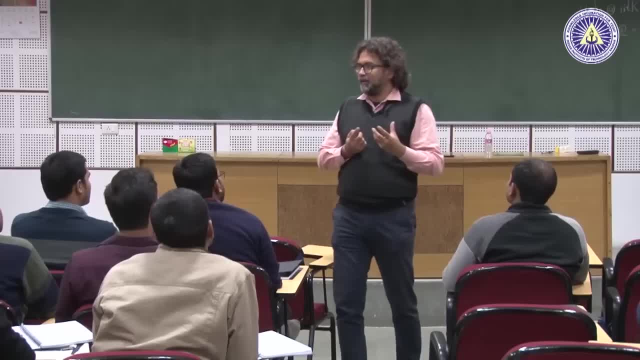 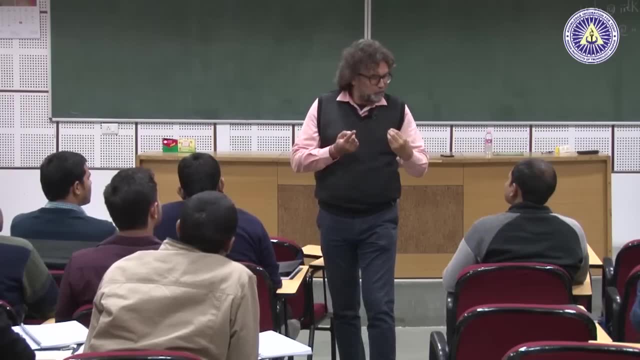 can take it as a semi-infinite type of an object, Is it not? And then the heat comes in, the temperature rises. ok, Now there is a pain threshold beyond which you start feeling uncomfortable. So now, as a transport engineer, or a transport engineer, you can. 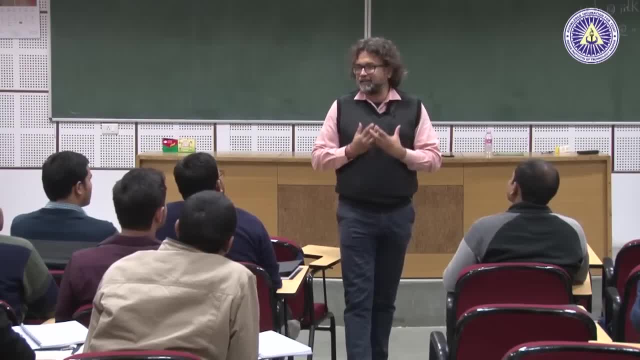 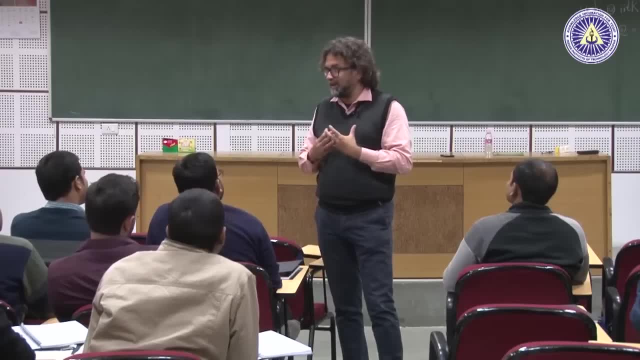 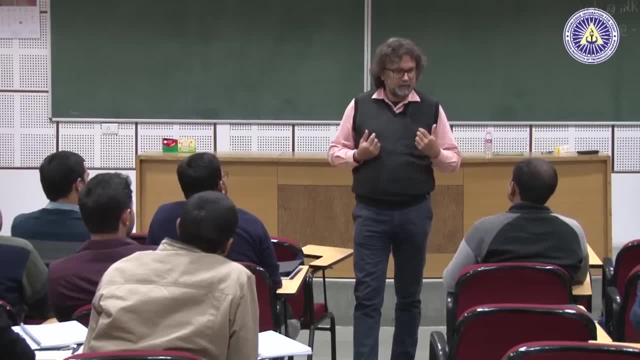 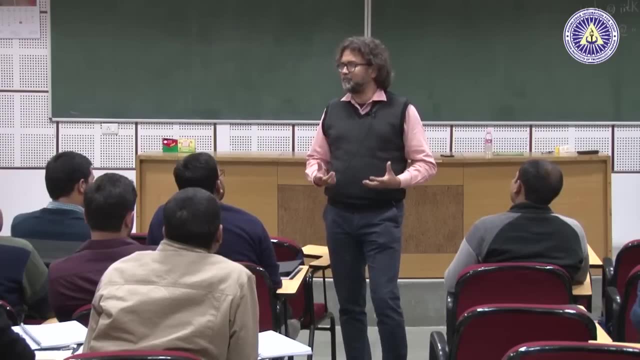 isn't it? You want to preserve the heat. You don't want to take it out, Isn't it? So what do we do? Forget about books, Forget about everything else. What do we do when our finger gets burnt? Ok, We can just keep it like that. We don't do that, isn't it? 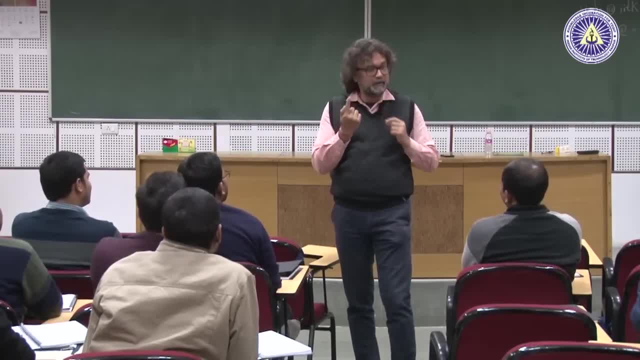 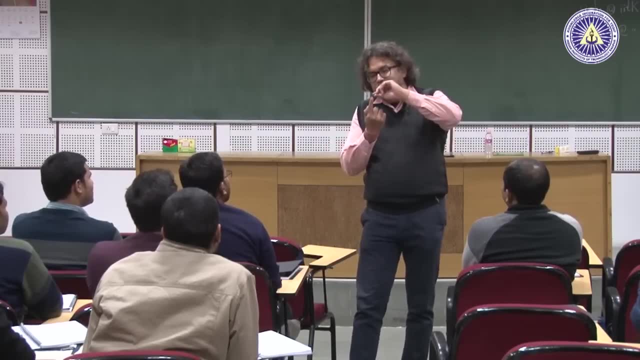 We can, It will cool down. Will it cool down or not? Yes, it will. It will cool down. We can just keep it like that, and there is a certain physics by which it will cool down, Is it not? Because the temperature close to the air, the air which is close to this finger, will get heated. 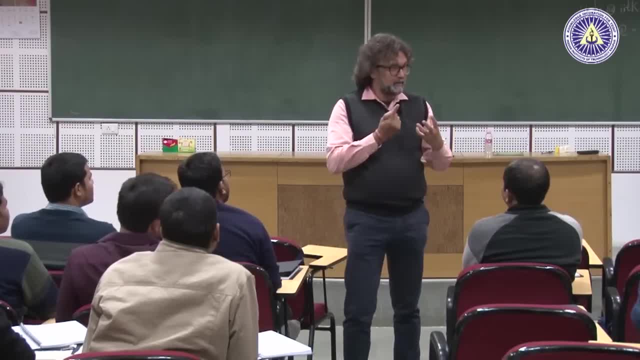 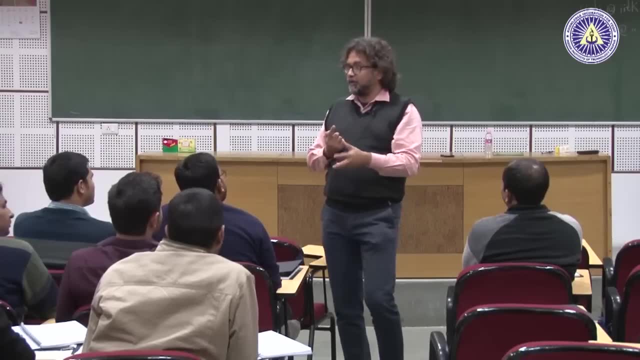 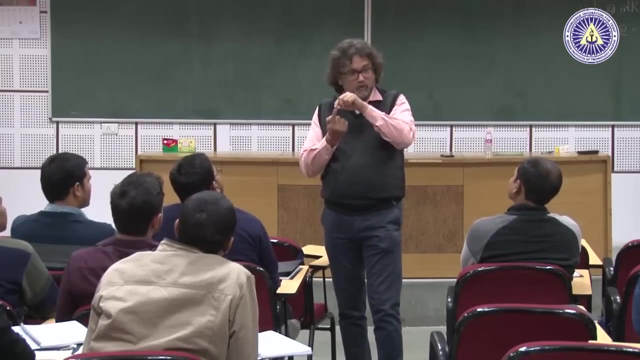 up, It will expand. There is a beta, Isn't it? There is a volumetric expansion coefficient. For an ideal gas. you can find it out. For a non-ideal gas also, you can find it out. It will expand. When it expands, it will become lighter. There is a buoyancy force, now rho. 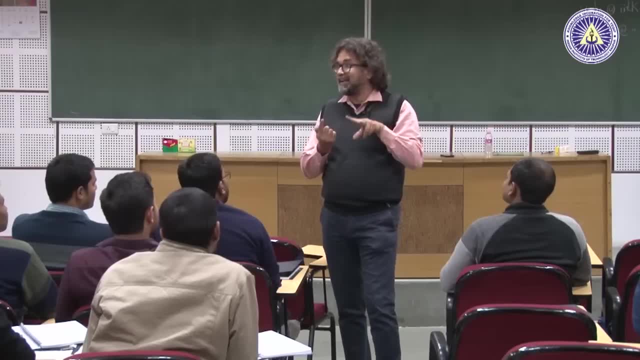 at temperature T1 and rho at the ambient. So there is a delta rho, So g times delta rho will be a force which will act on the object and it will rise. When it rise, cold air will come in, Isn't it? Now this can be formalized in a book and you can talk about. 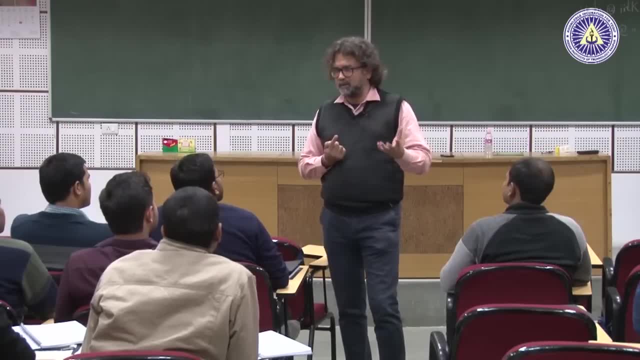 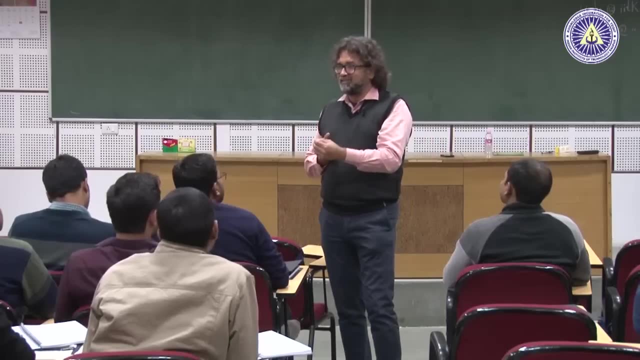 Grashof number You can talk about. you know Nusselt number coming out as a function of the Grashof number and things like that. Is it not That all formalization can come? But the student should understand that this damn Grashof number he already knows actually. 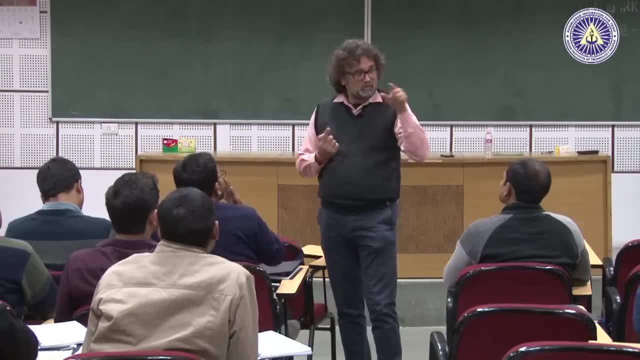 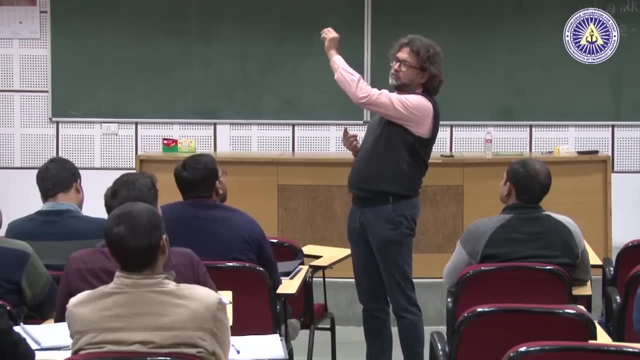 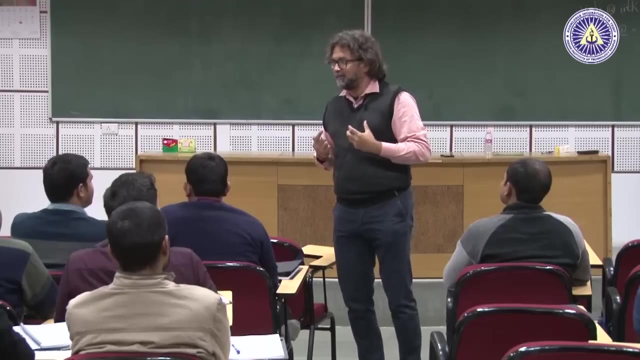 He already knows that it can cool down and this is how. So this is where your role as a teacher comes in. If you just derive, Nusselt is equal to constant in Grashof, to the power a. you know it will not click, It will not. the student will not become happy to learn. 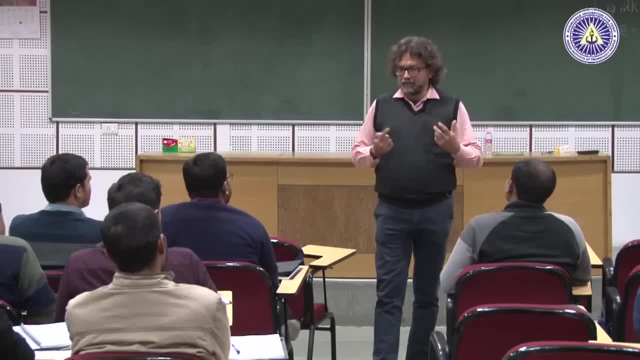 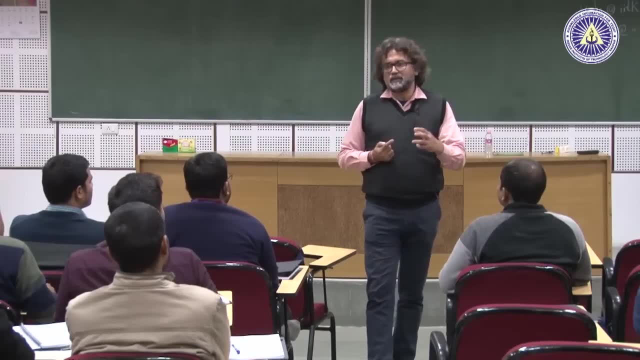 And then you will say: attendance is there? No one comes. Why doesn't he come? Because he doesn't get anything here, Is it not Cool, You understand? So the value addition which you guys have to do is the connectivity of 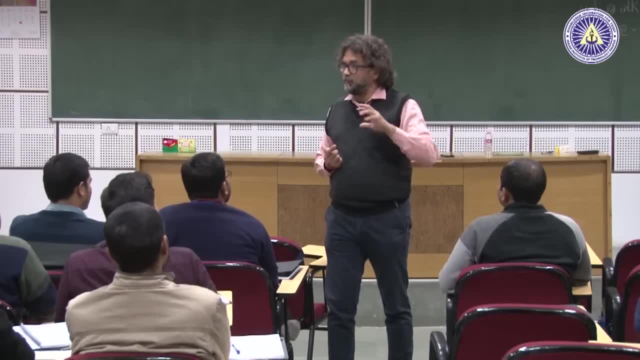 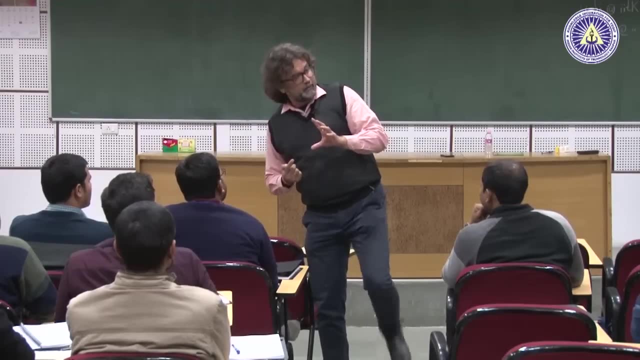 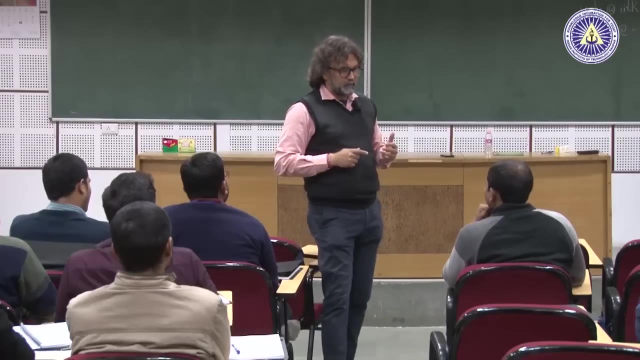 that equation with the outside world which we, they already know. actually, Even a dog knows that when there is, when his finger gets burnt, when his leg gets bent, he will do like this. So dog knows that if you do like that, the heat transfer increases Is. 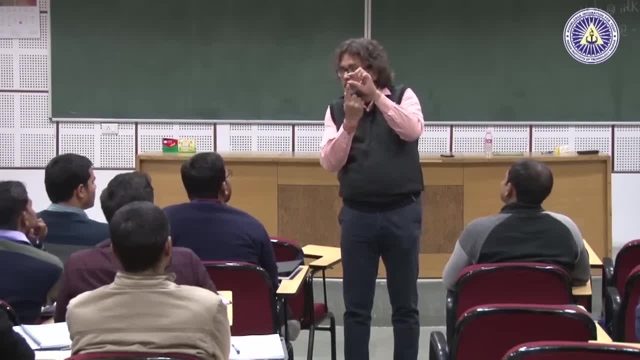 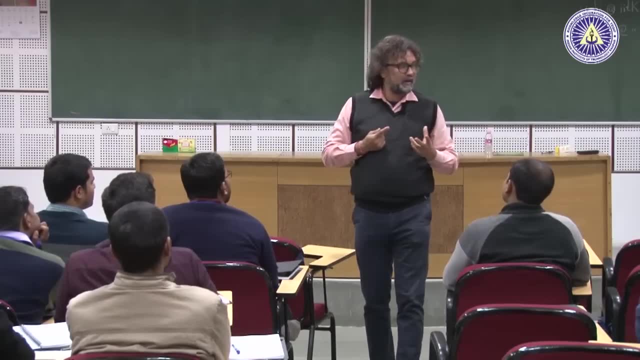 it not Why? Because just keeping it like that, the force which was there was only buoyancy. Now there is an inertia force, There is a relative velocity between the finger and the ambient, And then suddenly it comes that Nusselt is proportional to Reynolds. 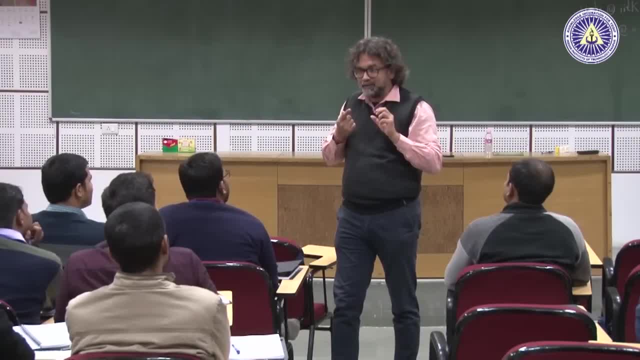 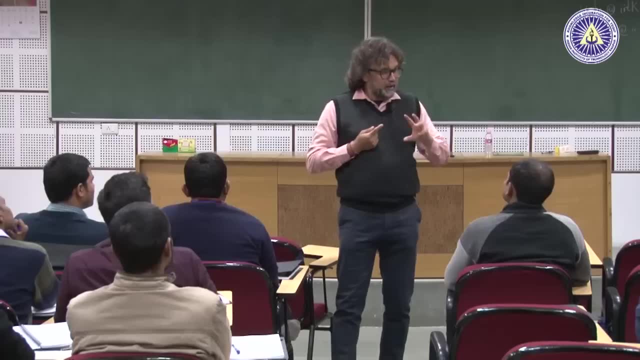 Isn't it? You do this, Reynolds number increases, Is it not? And then, yes, this is better, Is it not? If not that, then what do you do? You put it into ice, You put it in cold water. 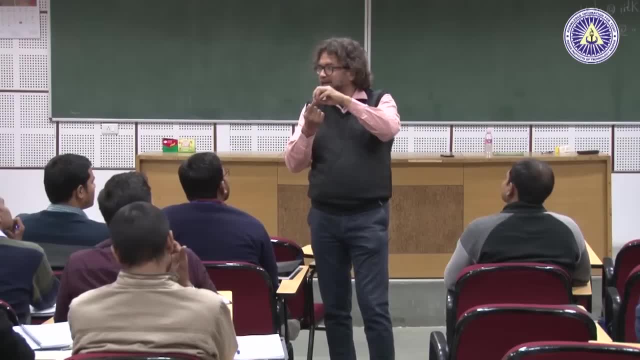 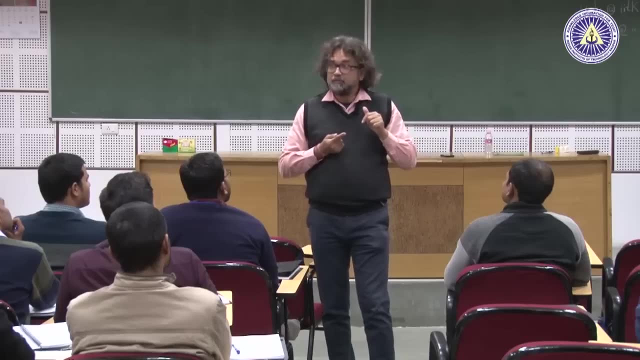 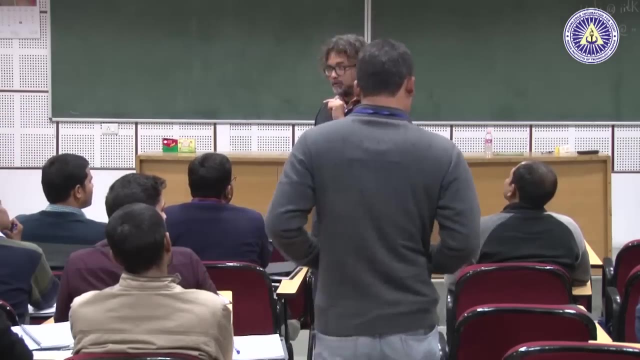 So that means previously some, some air molecules were hitting this, Is it not? Is it not? Now some water molecules are hitting it And you feel better. Even if the Reynolds number is the same, even if you keep the Reynolds number same, still you feel better. 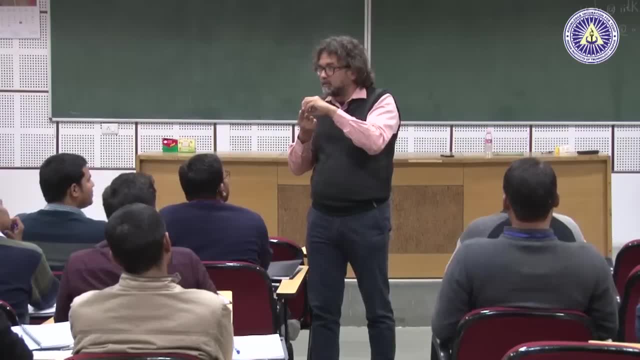 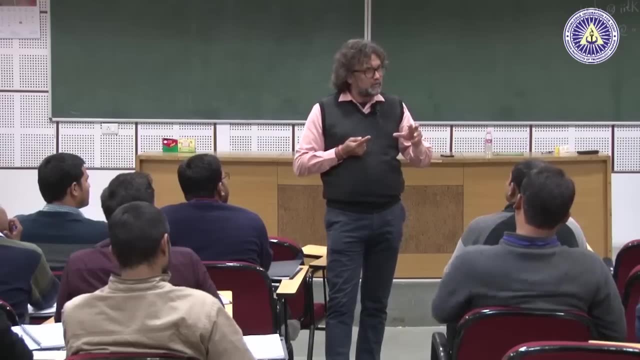 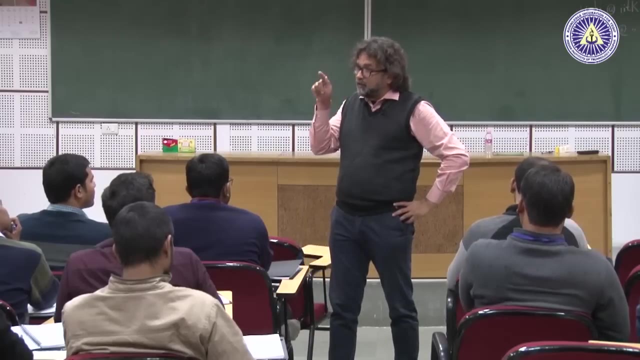 Because now the, the molecules which are hitting, they are, they are. something has changed, Isn't it? Something has changed. Now, the same molecules. when you change the molecules, your cooling curve is better, now, Is it not? That means other than the Reynolds. 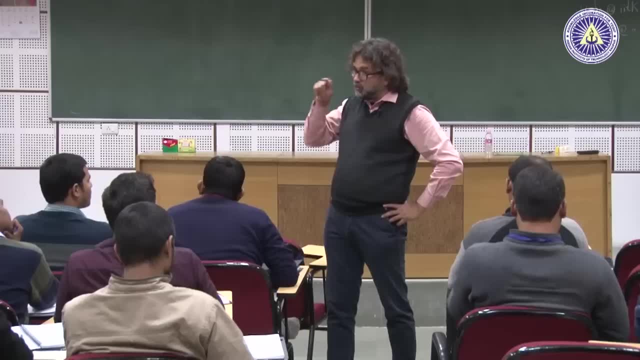 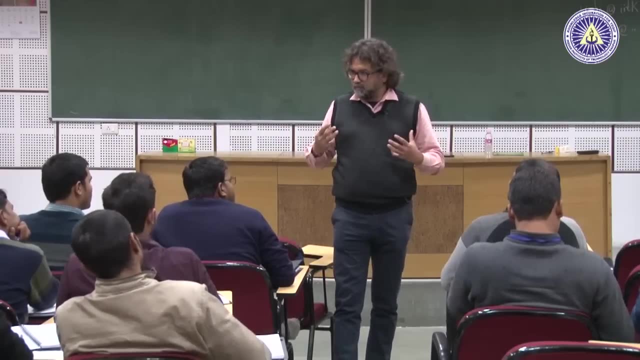 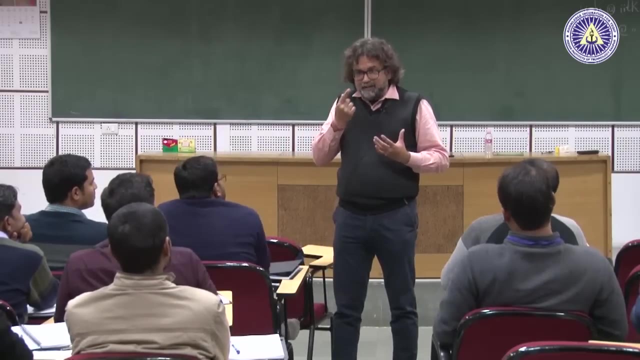 number. there is something else which has to do with the molecule itself which is responsible for enhanced heat transfer, Is it not? Do do you agree with me Then? now, suppose you are still not comfortable. What do we do? We put we make it wet and 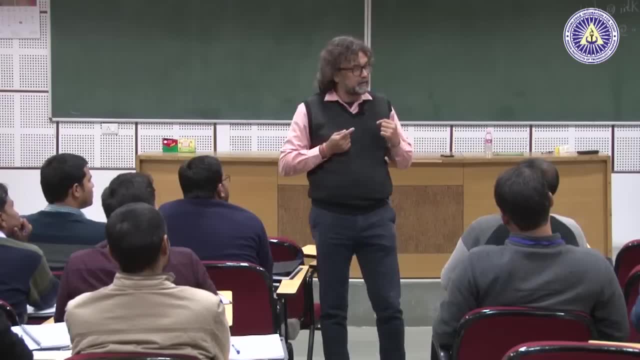 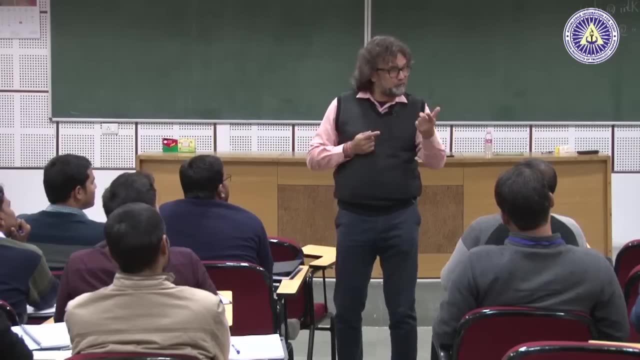 then blow air. Now it is much better. So what have we done? We have changed the physics. now, From single phase heat transfer we have moved to two phase heat transfer. We are now making use of the latent heat. The HFG was not there in the previous example, Is it not? 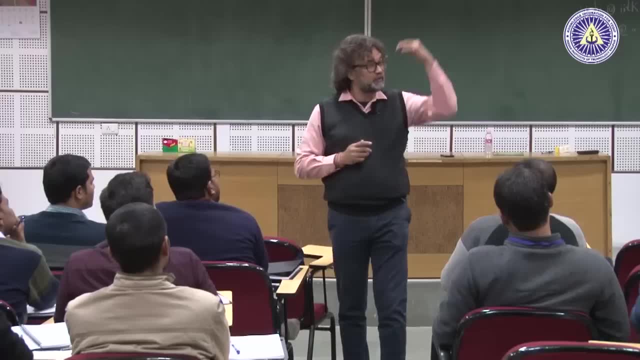 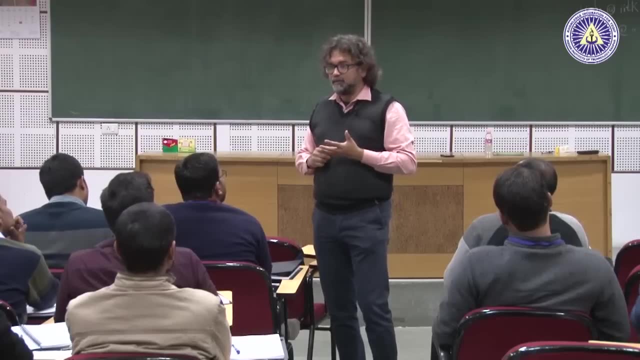 Now latent heat has come in And we suddenly see that the heat transfer coefficient is now much, much, much better. If you put some ethanol, you know, and then do like that, that will be still more better, Is it not? So this is where you, as a teacher, have to. 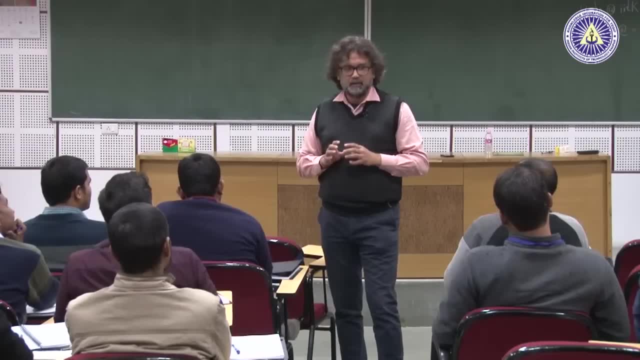 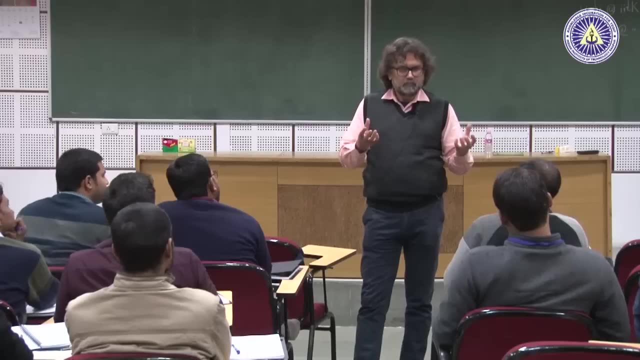 come in. Okay, You, as a teacher, have to come in, For example, all heat. for example, your mother, you know, when she she cooks aloo, Is it not Aloo ko jab ubhalte hain? then what do we do? She keep, she keeps it on a. 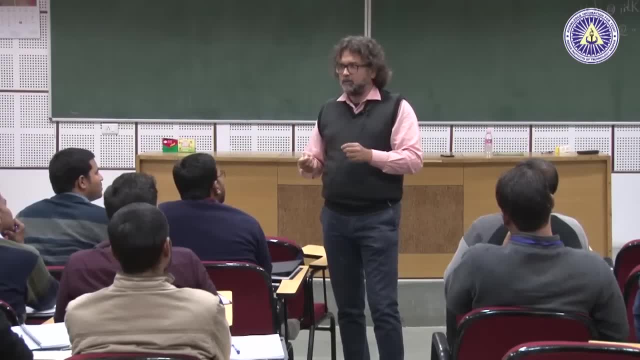 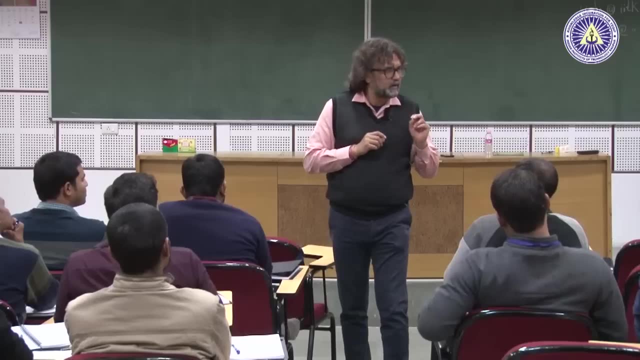 tap water or paani mein dal ke, and then she starts peeling off. So the temperature must be the. the temperature of the top surface must have come below 40. Otherwise toh haat jalaega 40,, 42 ho gaya hoga, Is it not? After that toh haat jalane lagega. How about the? 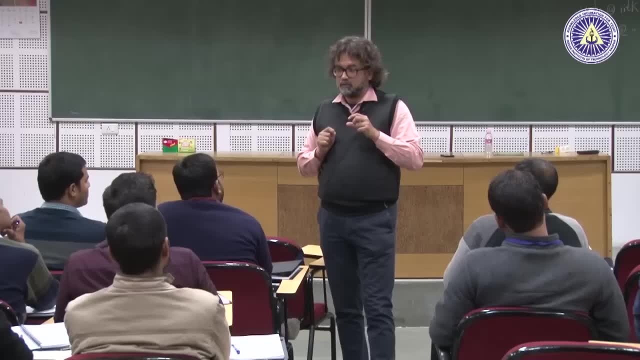 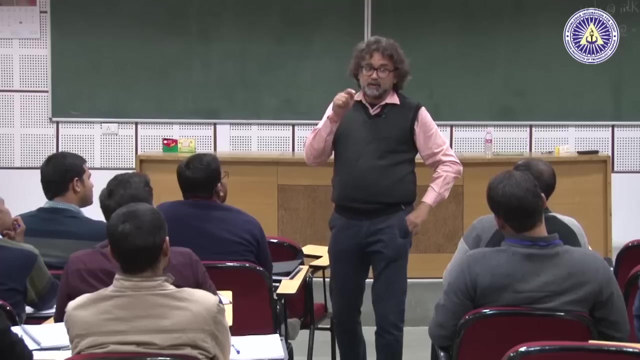 inside temperature. Is it still 100?? Is aloo inside also hot enough? When the temperature when the peeling takes place, What The temperature outside is 40,, 42.. What about the inside temperature? If you break it open, you see steam. you see steam. That means can you take aloo as a? 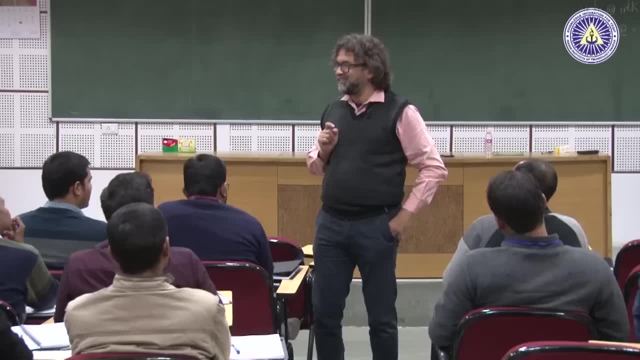 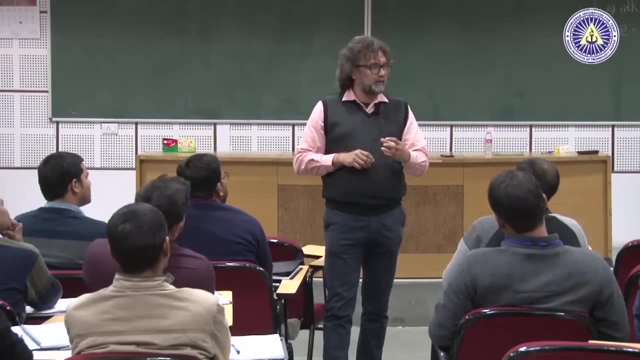 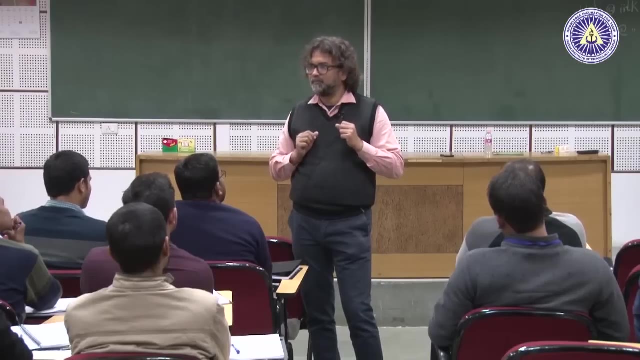 lumped parameter system. No, you cannot, Is it not? Is it not? If you have a copper ball and if you put it in water, isn't it? What will happen? The inside temperature and the outside temperature will be more or less the same, more or less the same, more or less the. 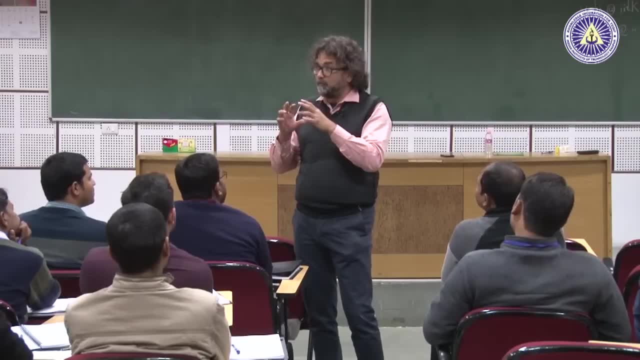 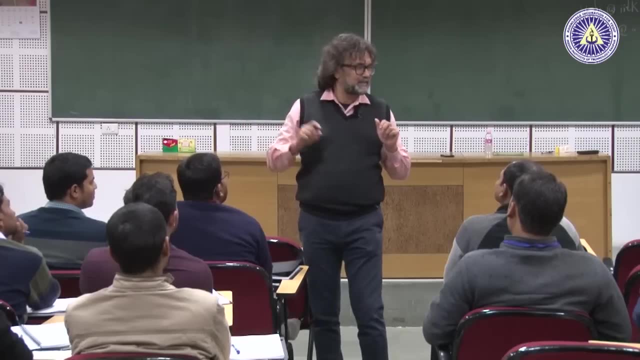 same, isn't it? So now you can now with this, with this discussion. then you say there is something called B O number, There is a thermal resistance of conduction, thermal resistance of, you know, convection, and then you describe: what is the numerator, what is? 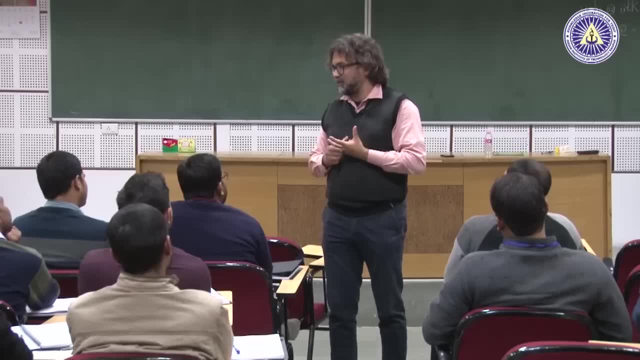 the denominator, and then it will come alive, Is it not? So I mean, we take bath, for example. you know when we take bath. if you just put it in water, you know it will come alive. So I mean, we take bath, for example, you know when we take bath, if you just put it, 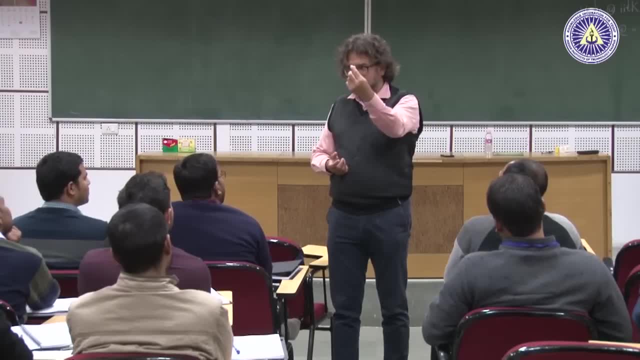 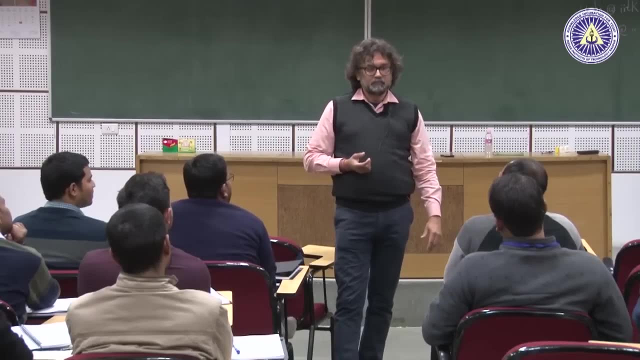 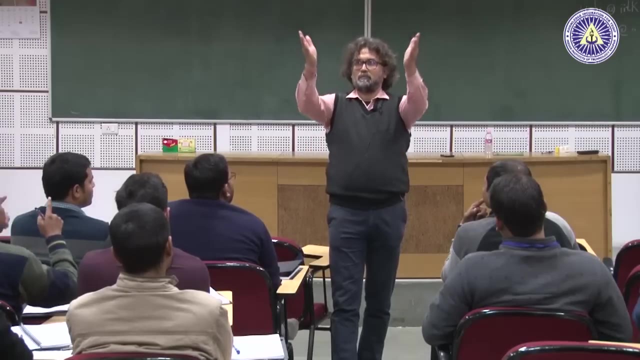 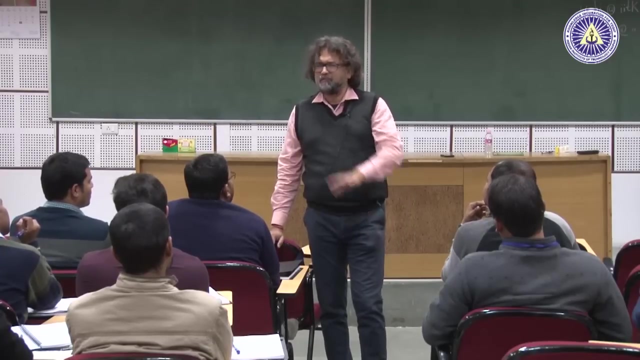 in now. Yes, we put another bath, we put another 1.. Well, in a method of conversion of water, let it do some thing that it will come in the same size. then the bath is not very small. No, Like a, like a form, ikkegrade. 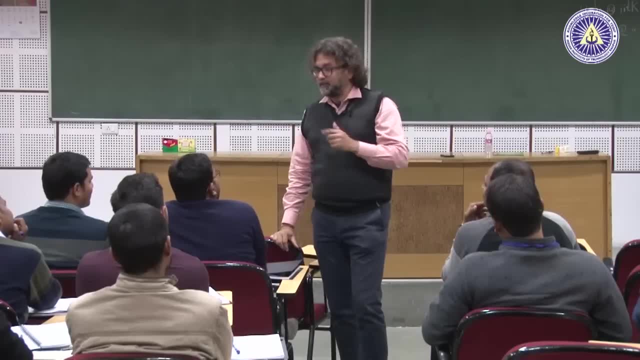 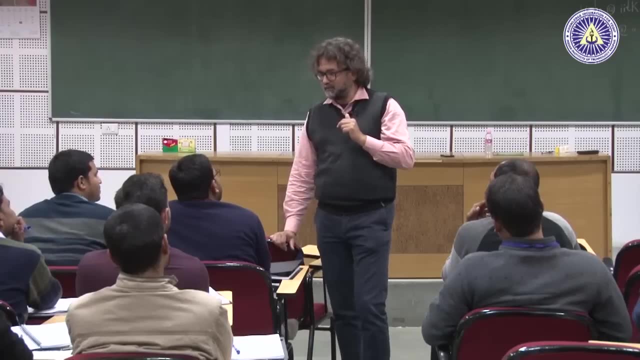 No forget formula. ya, Peter, gracias murar pi. No forget formula. ah, forget formula formula at the end. first understand it. Speed is increasing. Speed is increasing, that means it is accelerating and rho a v has to be constant, it is a. therefore, you will see that as the velocity increases, the area of cross section will go down. After a while it becomes unstable, and then you can get small drops, is it not So? who is supplying the energy to give the drops? because surface energy is needed to create drops. who is supplying? 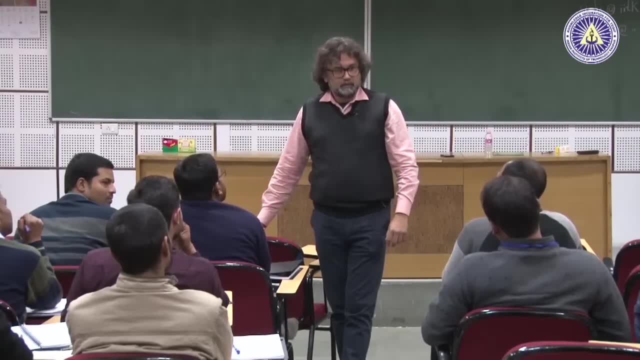 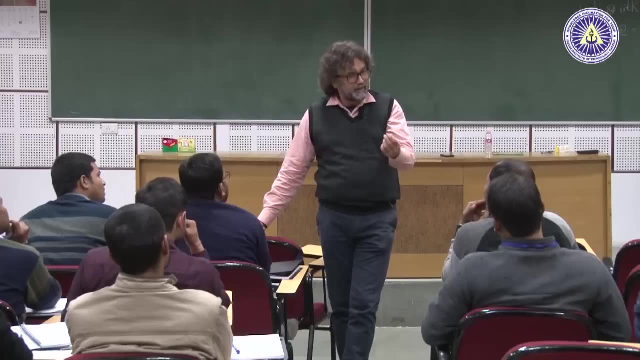 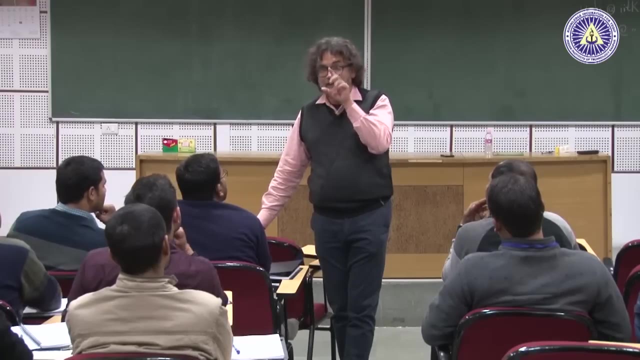 that energy. So the kinetic energy, the inertia of the system, the kinetic energy, the accelerating kinetic energy, the gravitational pull is there and that kinetic energy part of it. but why does it become unstable? Then you go into the, then you have a Navier Stokes. 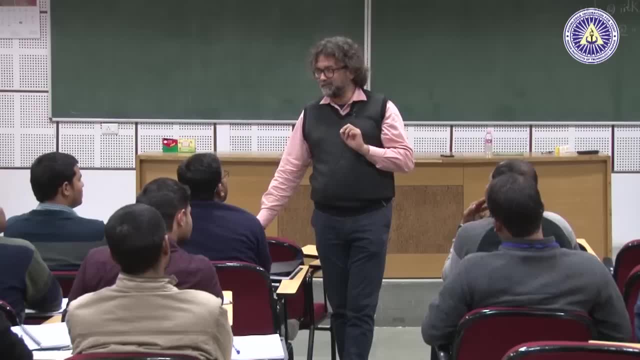 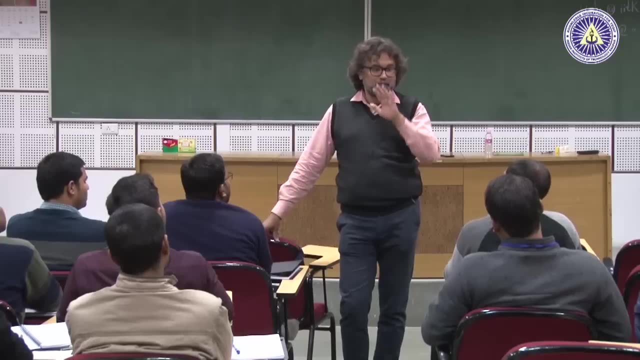 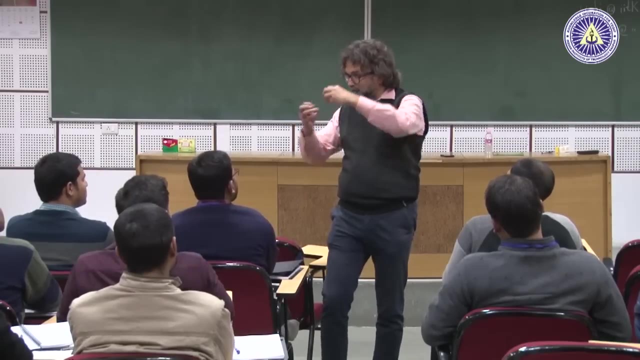 equation, you perturb the Navier Stokes equation, you create a perturbation equation, you subtract the two and have a linear theory, for example for perturbation. and then you will come to know that there is some Rayleigh Taylor instability. There is some. there is some sort of an instability which will grow, and when that instability grows, 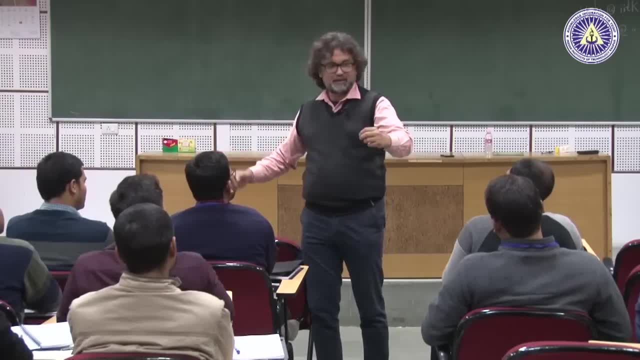 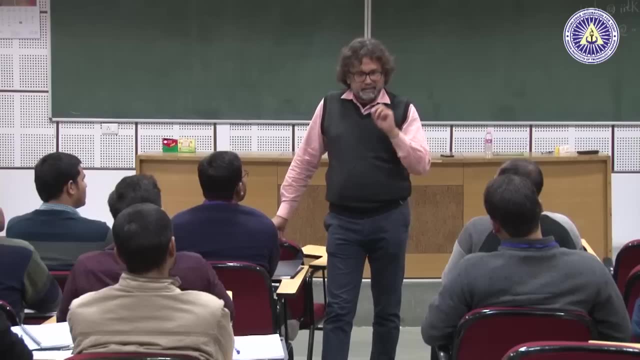 this nice jet which was coming will now break down, you know, and you will have atomization, for example. So what I am trying to tell you is very simple. what I am trying to tell you is, please, whatever subject you are teaching, whether it is thermodynamics or heat transfer, 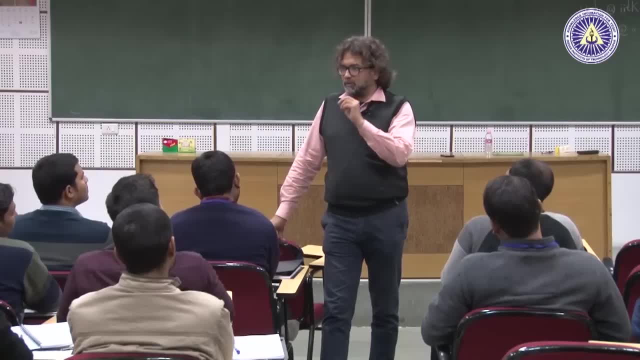 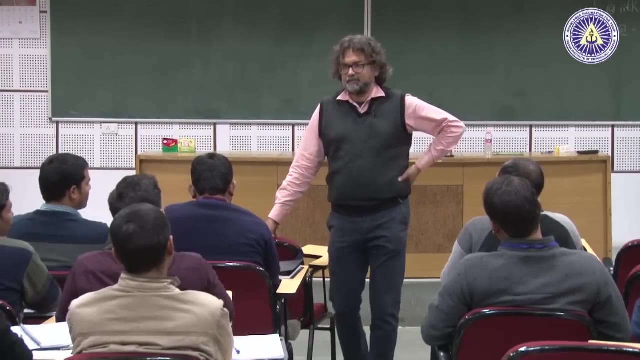 or solid mechanics, or manufacturing process or fluid mechanics. please see that subject around you. How many of you have heard of thermodynamics? how many of you have calculated the rate of heat transfer from human body? How much heat are we dissipating? Can the? can a problem be simpler than that? Every day, we dissipate. 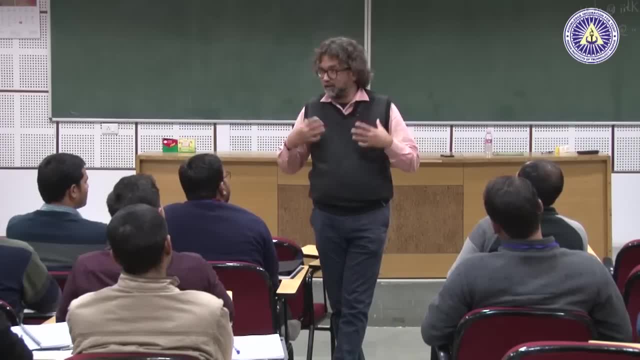 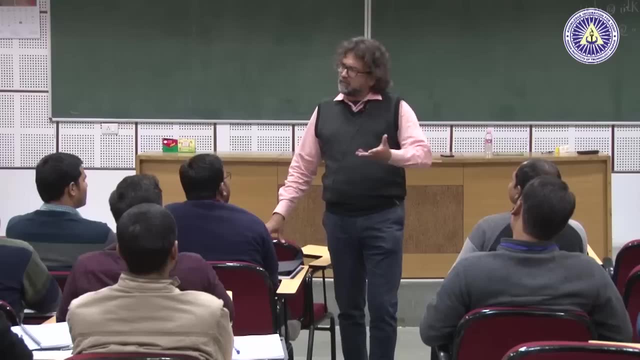 energy every day. we try to. right now, I am trying to reduce my energy as much as possible by putting multi-layer insulation, isn't it? This is MLI, isn't it? Multi-layer insulation? okay, How much energy are we dissipating? Anybody any idea? rough guess. 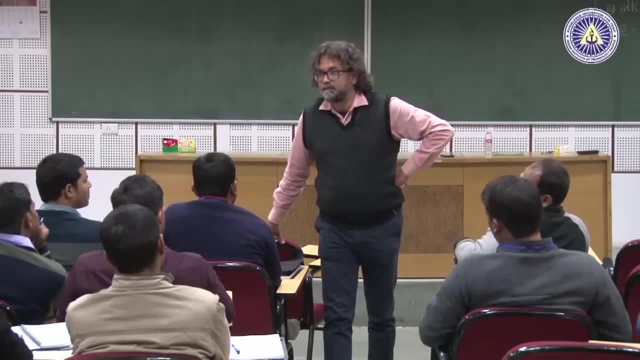 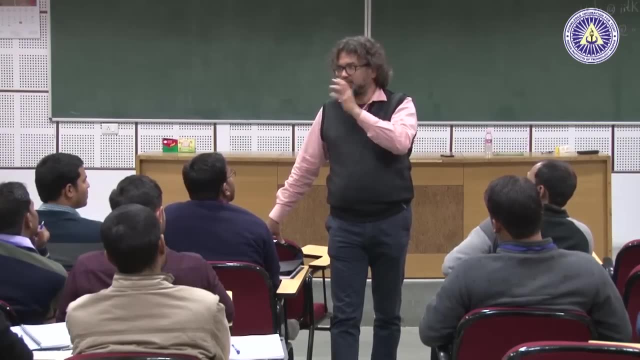 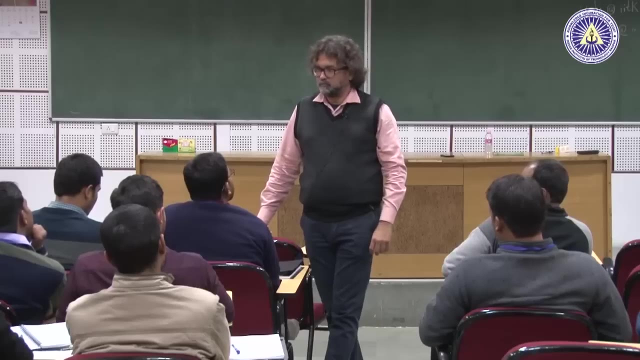 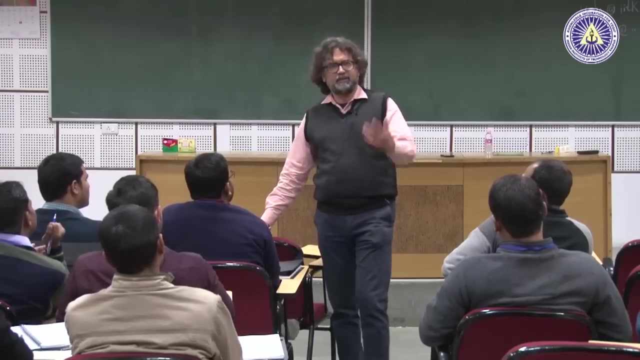 What 50 watts he says Around. okay, So that is the first guess which he has made Right. Let us say it is fixed. let us say, right now it is 25.. So delta T is 20 degrees. let us say: 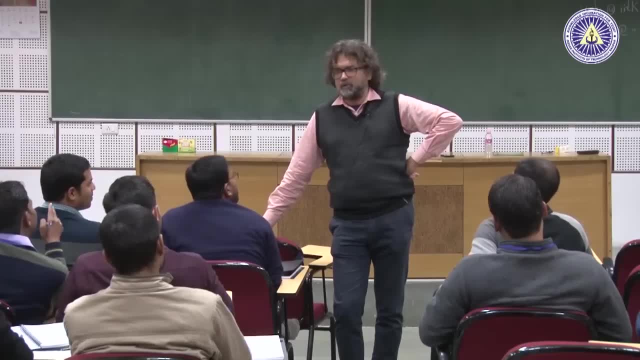 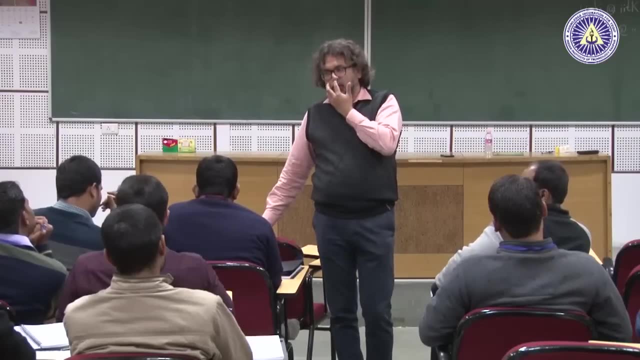 Yes, How much is the typical area human body area? We will assume that body as a cylinder, As a cylinder, that is a very nice model you can make as a cylinder, But forget about cylinder also. I can give you the area of the body also. no, you should. 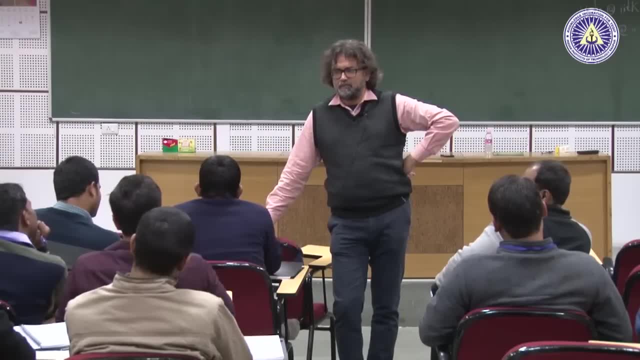 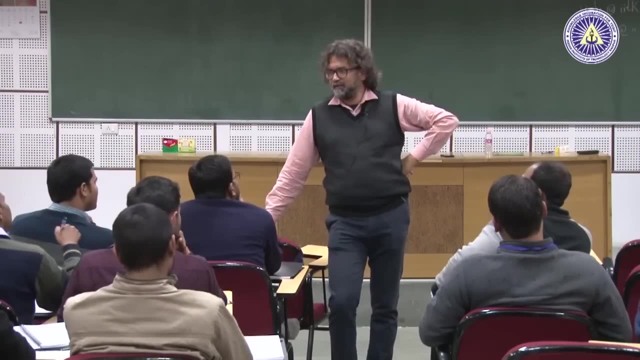 know the area. how much is the area of the body? Any idea grown up body. how much is the area? Any idea? A rough guess cylinder like: Yes, we can say sir, 2 pi R L. 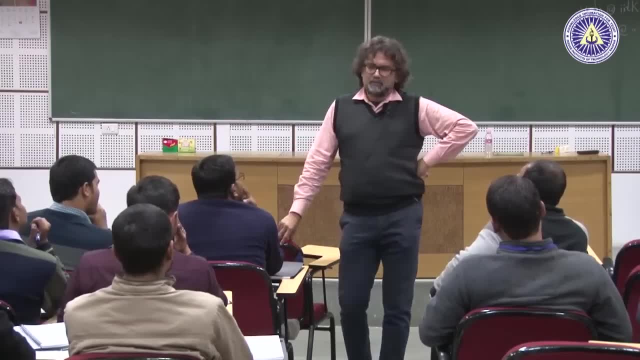 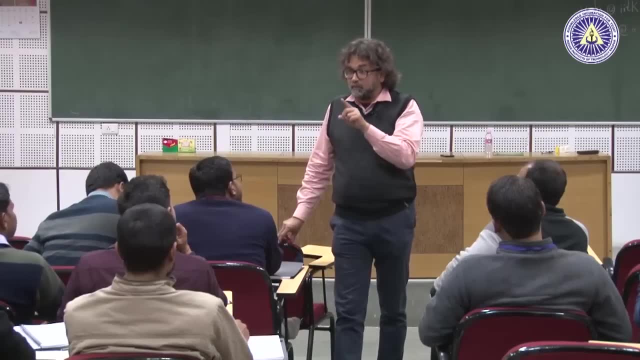 Yes, yes, Is it not? Yes, sir, So We will assume. So this is you know. I mean, I am not interested in the answer right now. I will tell you the answer. that is not. but what is important? 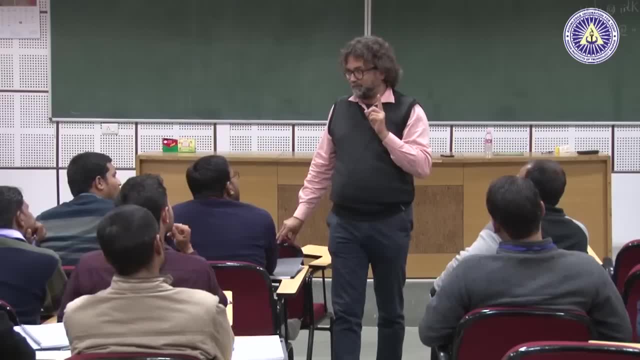 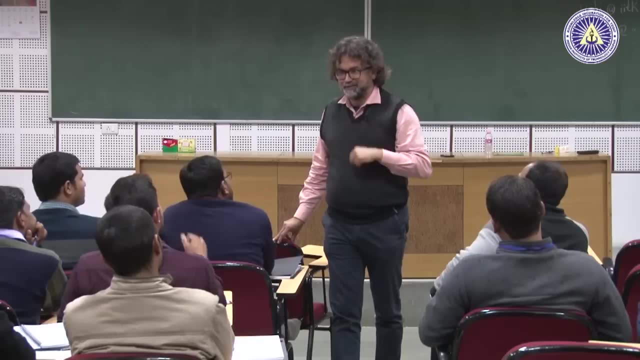 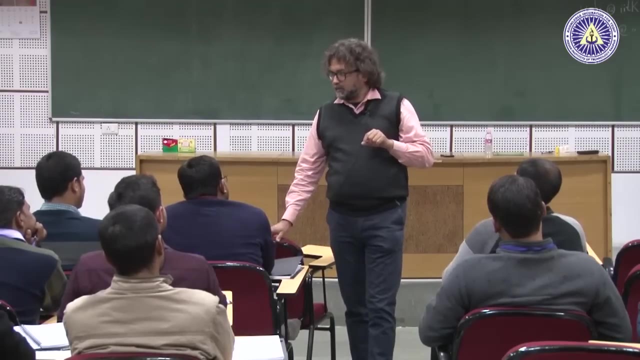 to know is that you have all M Tech, all have studied heat transfer, but we have never bothered to calculate how much heat is dissipated by me, is it not? This is what I am trying to tell you. you understand. You know how to do a differential equation, you know what? 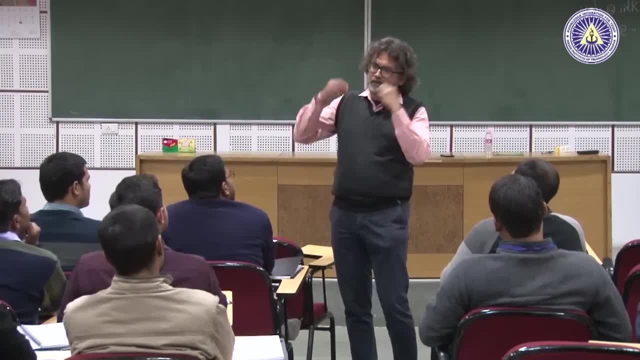 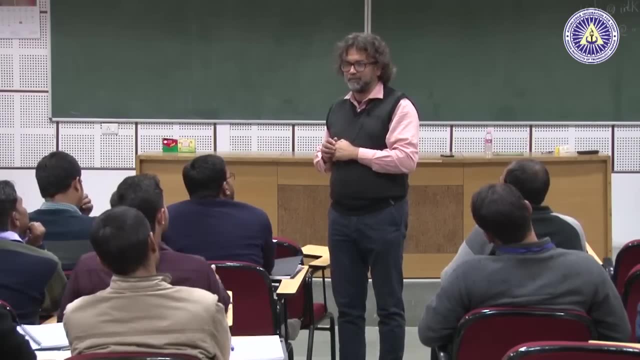 is homogeneous equation. you know what is non-homogeneous equation. you know what is non-homogeneous equation. you can derive, you know you can, if the boundary condition is known to you. you can get C 1, C 2, you know, and get some. you know some values. 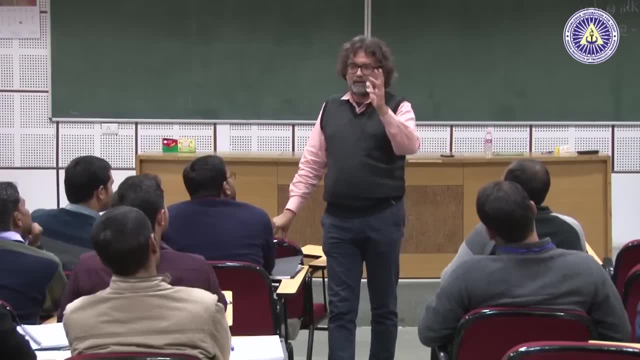 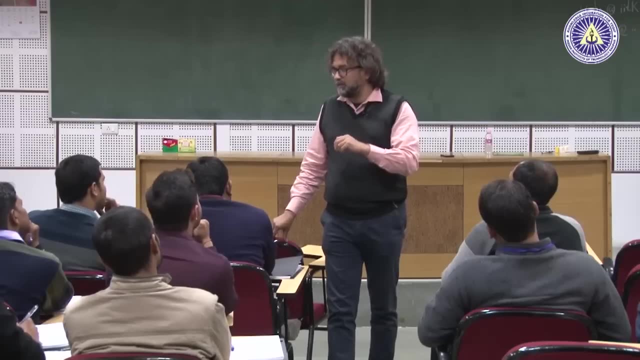 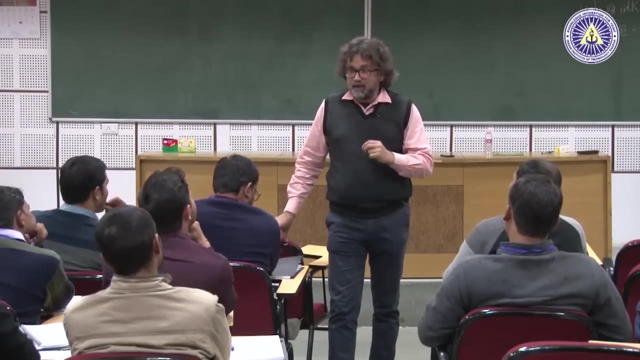 of the constants. ok, You can convert, you know you can have some, you know separation of variables and integrate all that you can do, but the connectivity with real engineering is not there. that is where we have to be different and that is why I am different. that is what. 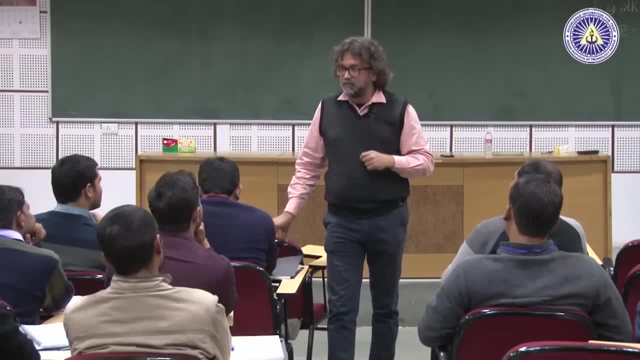 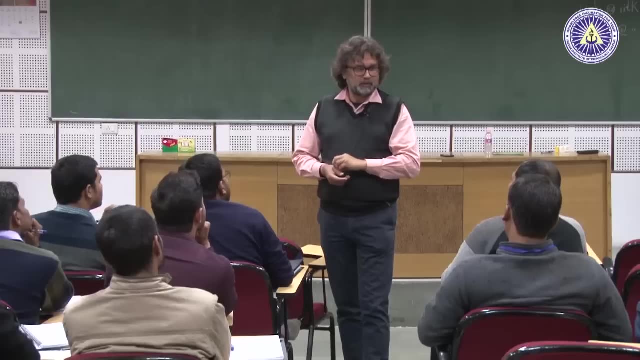 that you have to say also, after 5 years, that I am different because I make my students connect to the real world. you understand, I still remember my first interview was in ISRO, in a campus interview, ok, and I entered the room, you know there was this door and 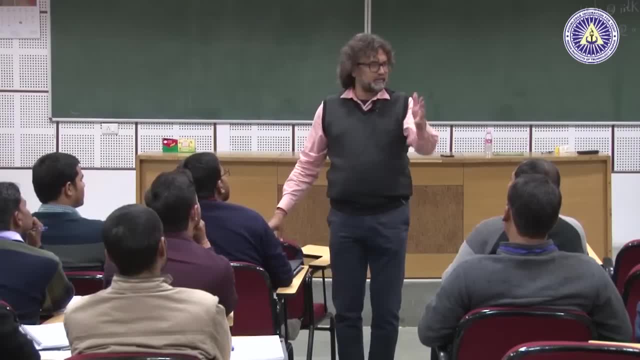 I pushed it and I entered and I sat and then, after some discussion, the person asked me: please tell me a example of combined loading. ok, Now, a typical description is that you have toned the temperature. you have toned the temperature. 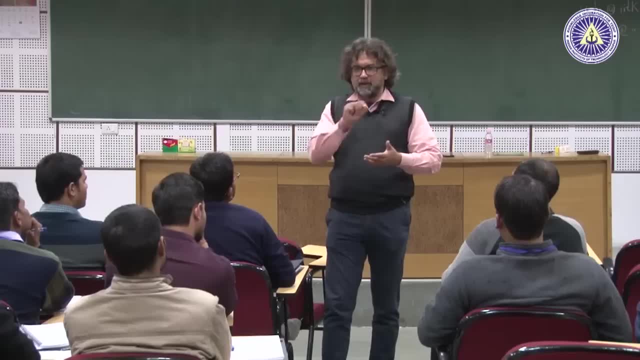 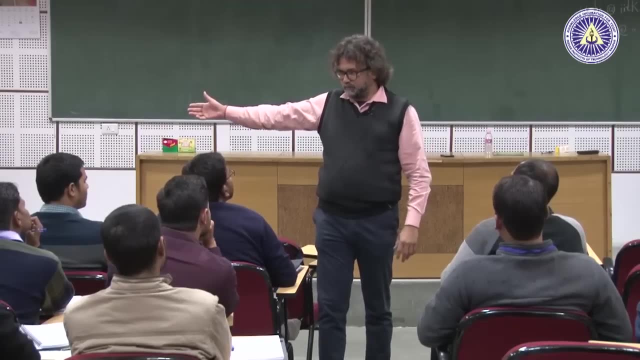 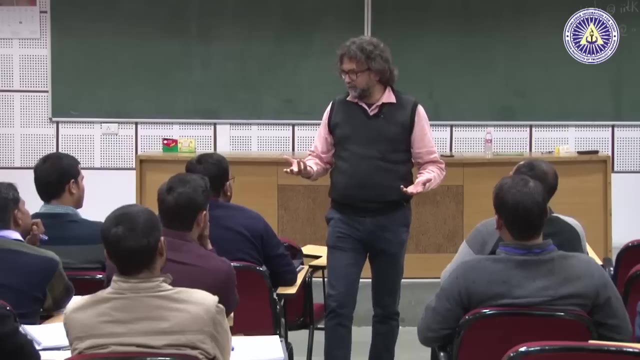 Ok, typical student will start thinking: combined loading means: beam banayega uske upar kuch karayega. point load, this load moment. I just told him that I just entered the room. the handle I had to give a torque and push combined loading, is it not? This is what I want you. 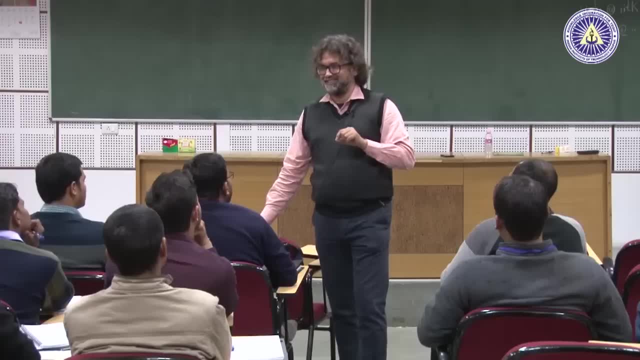 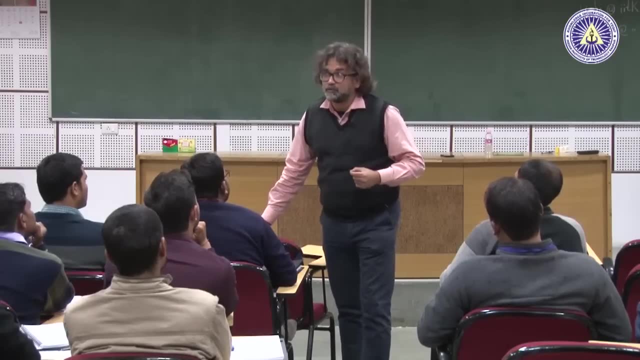 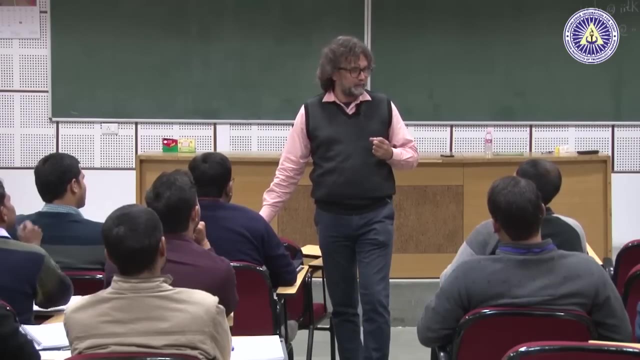 to do and then you will be a good teacher. you understand, The student must be enthusiastic enough after your course that as soon as he starts going out, he starts looking everywhere. kaha fluid mechanics, dikh raha hai. mereko. kaha heat transfer, mereko dikh raha hai is. 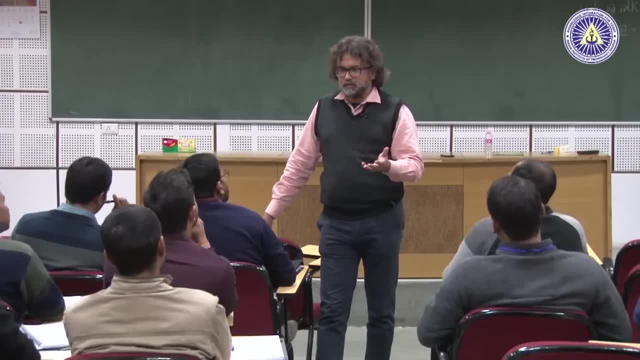 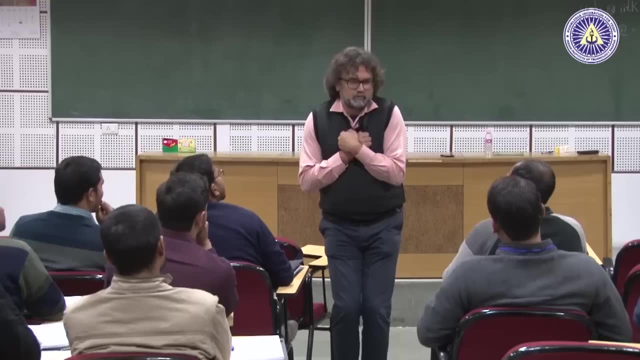 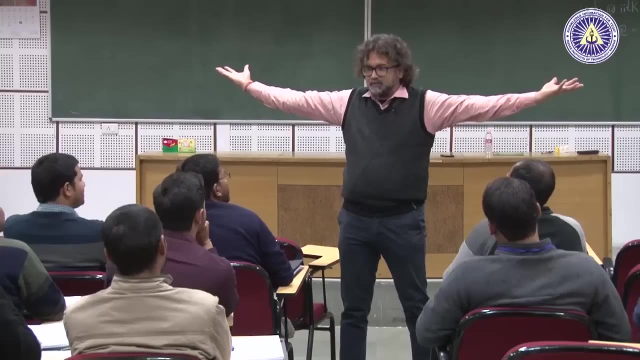 it not Extended surfaces? fins we teach, is it not? we see fins everywhere, is it not? Whenever we are feeling cold, we sit like that. when we are not feeling cold, is it not? garmi hone lagta hai. So is it not finning system? am I not extending my area? 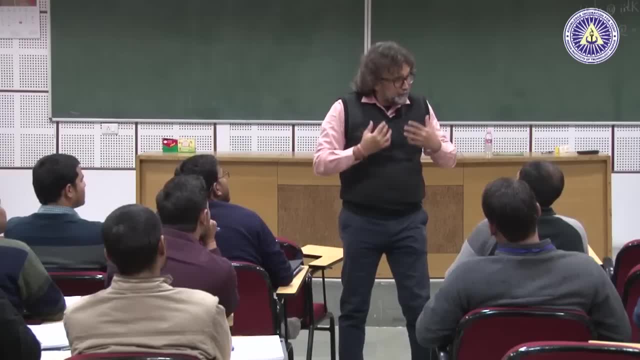 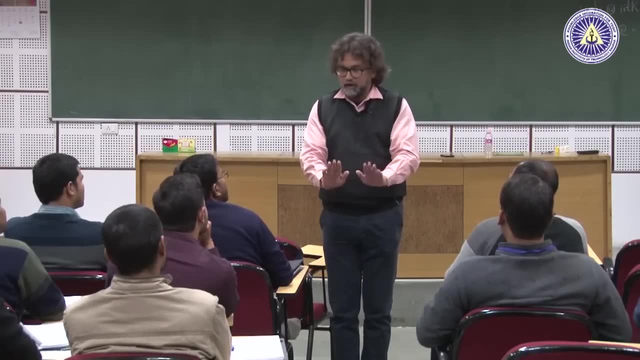 Is it not So? why don't you take this as an example? Jab mereko thandi lagta hai toh mai aise haath karta hoon usko, if there is a fire here, I don't put hand in line with. 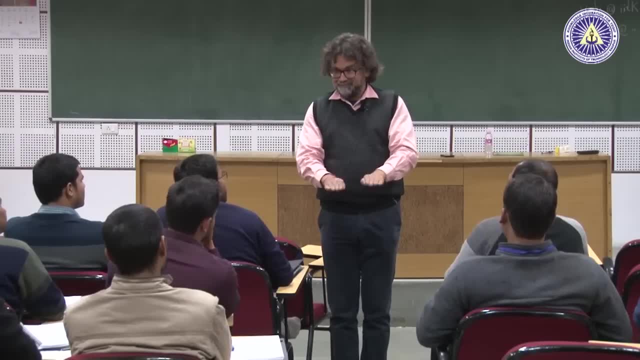 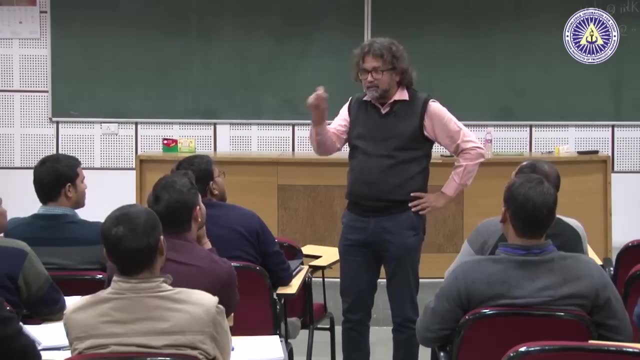 it. so there is a shape factor, Is it not? Aise aise karta hoon dheere, dheere garmi badta rehta hai mera Toh shape factor ke liye, wo chitra bana ke omega area, wo baad mein karo. 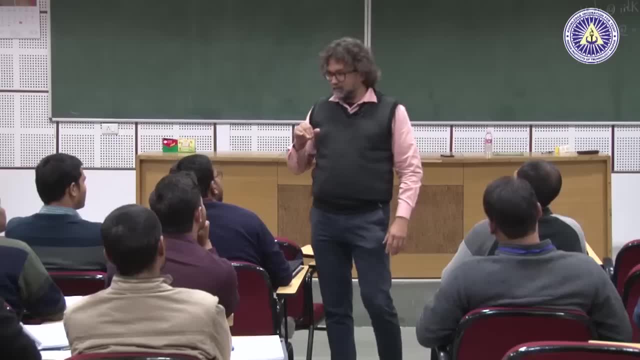 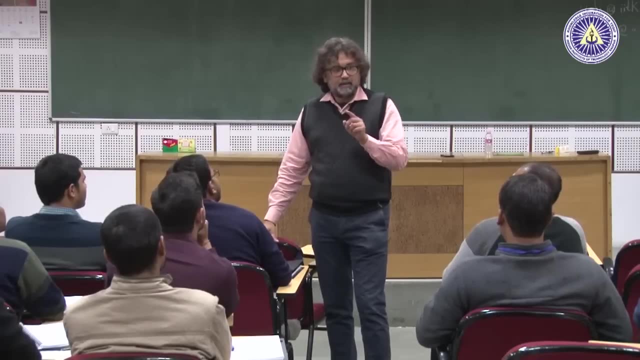 wo karna hai? I am not undermining it, I am not saying that you do not have to do that. You can't only talk. they have to analyze also, they have to understand. But then which equation to use when? which boundary conditions? 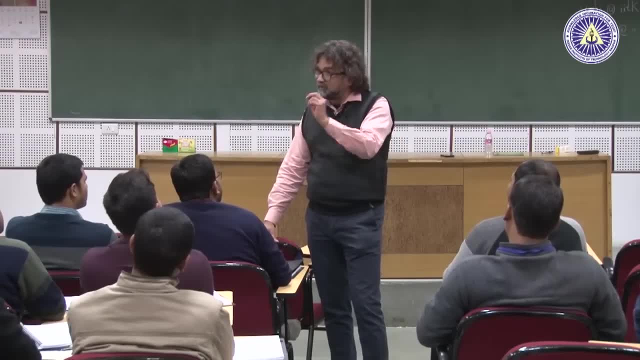 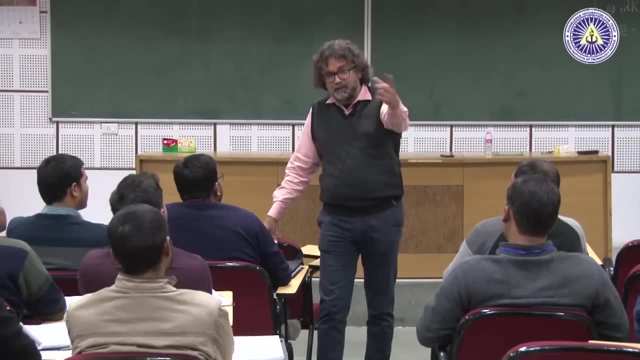 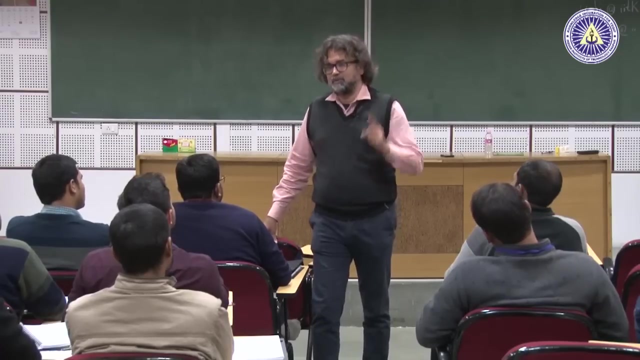 to apply which? what are the assumptions under which this equation will be valid? Okay, and the spark which comes that, Oh, this can be solved like this, Can only come if the teacher has done the due diligence that he has made his students of the connectivity of that equation, the terms of that equation, with real-time situations. okay, 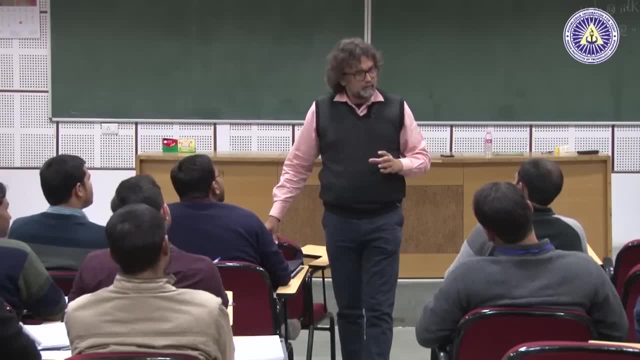 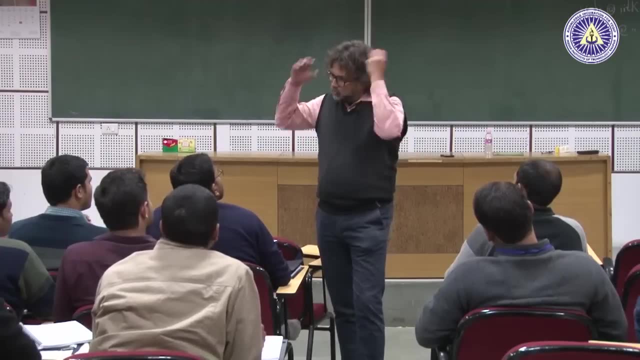 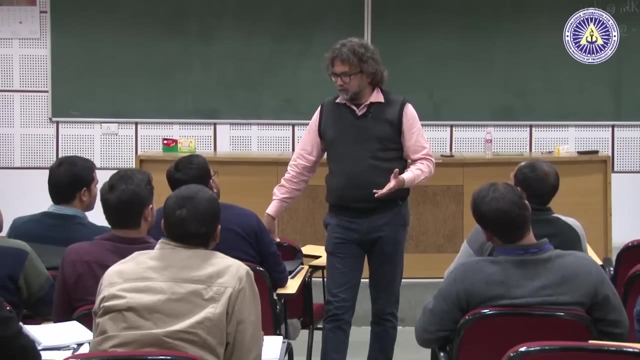 so if you want to do it, it's it's. it's hard work. it's not easy. see, right now, what has happened is, unfortunately, those people who don't do don't get anything else in life. they want to become teachers, when we are all part of the same community, is it not? but then once, fine, that's also fine, you'd. 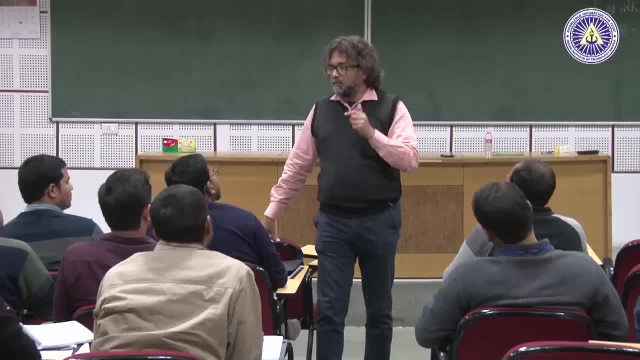 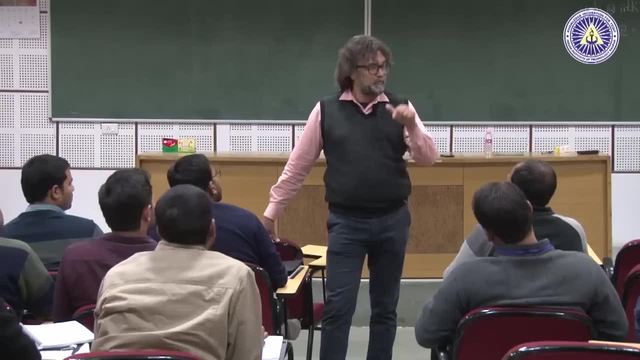 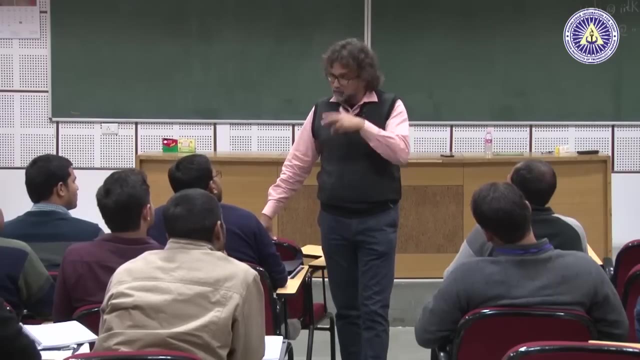 never got anything else. now you want to become teacher. that's also fine. but once you want to become a teacher now, then everything which is needed to make that profession worthy of it and you enjoy, your teachers, your, your students enjoy, your, your colleagues enjoy- is what now you have. 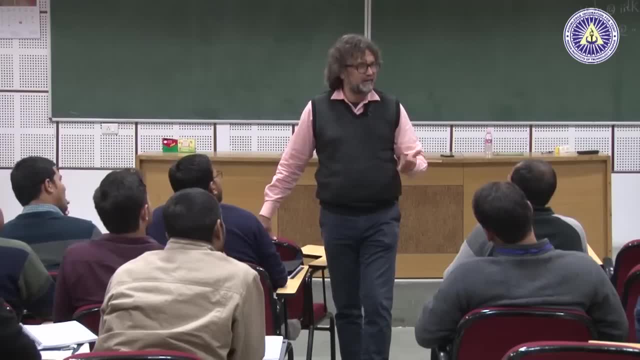 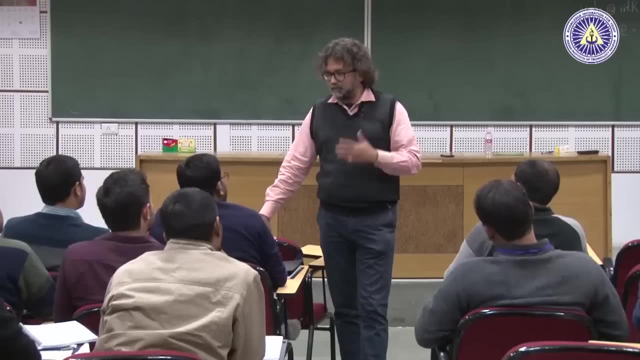 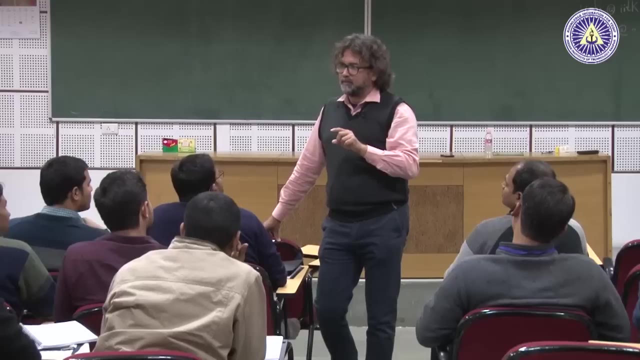 to do? you have to inculcate an interest. if the interest is not there, if the interest is inherently there, then there is absolutely no problem, is it not? absolutely no problem? okay, so coming back to that question, you know so is radiation important when heat transfer takes place from human body? why normally people? 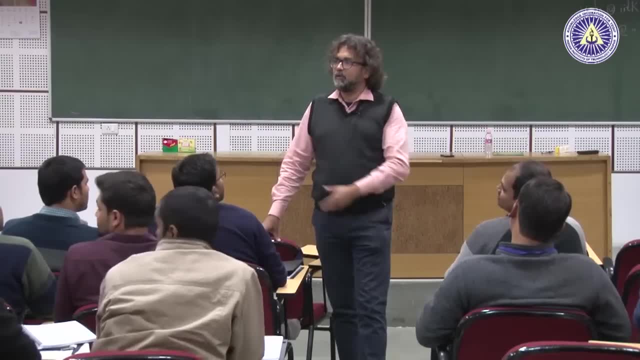 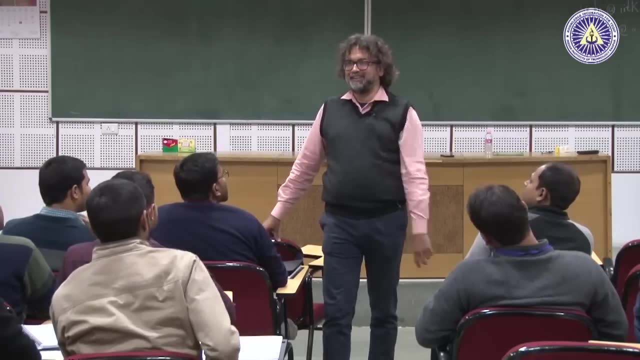 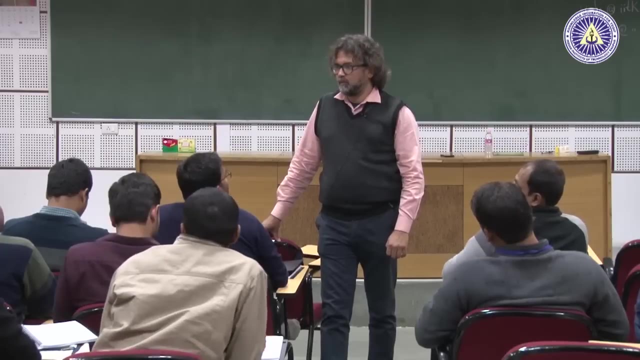 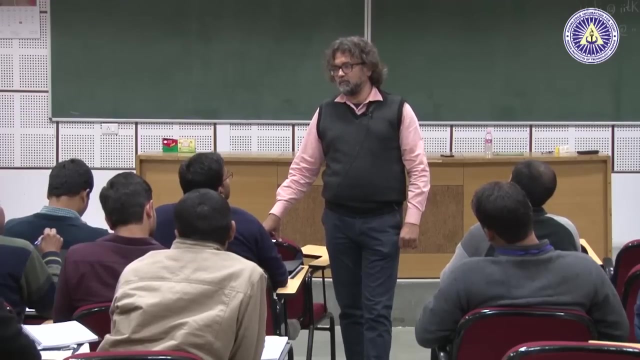 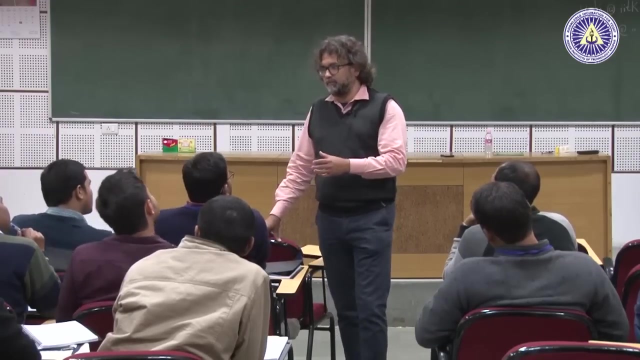 say that radiation is only important at high temperatures. we are not high temperature, so why do you say radiation is important? forget that. but how? why is it? why do you think it is an important thing? when you are you, when you are doing a human body calculation, if I am going on a motorcycle, I am doing a calculation for the 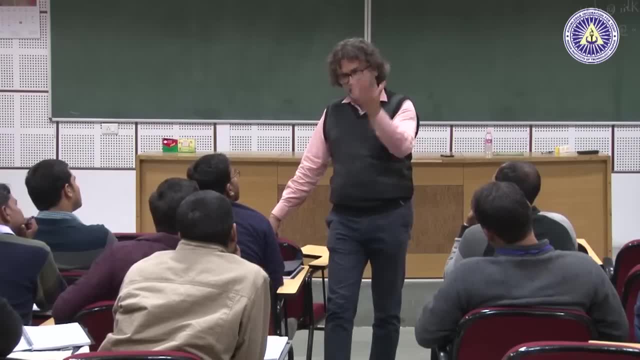 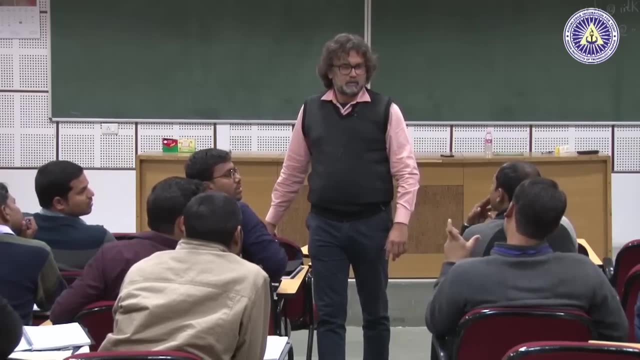 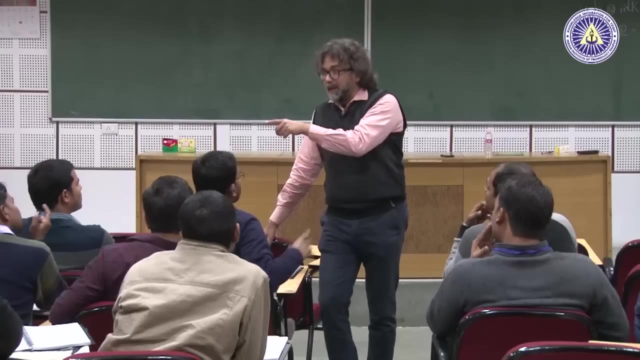 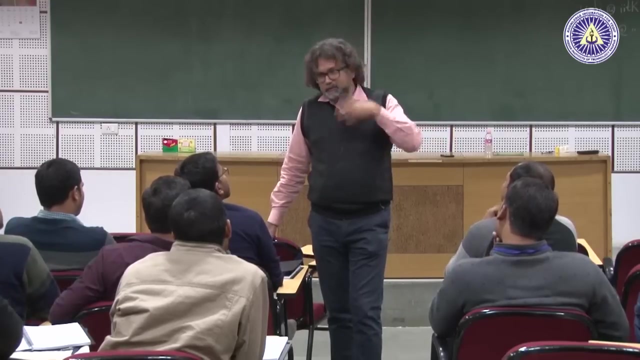 heat transfer from the engine fins, I don't care. radiation, the temperature is much higher than the, but at the human body, the temperature is only 37, what we know, yeah, comparable to absolutely. so what? so? the idea here is that there are several modes of heat transfer. okay, and all of them are probably. 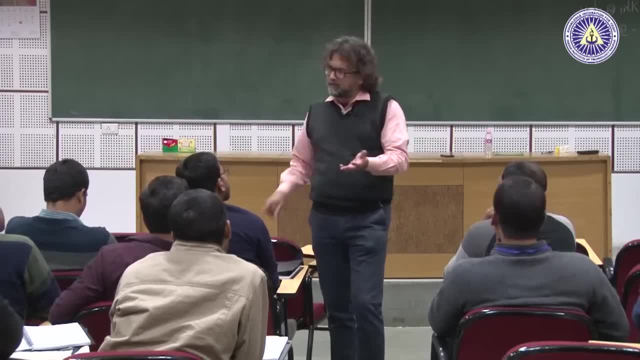 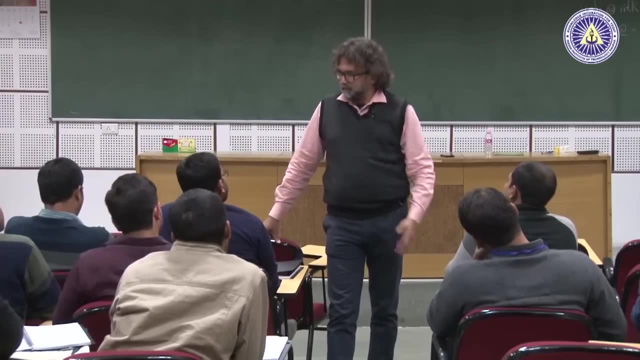 playing a role all the time, is it not? most of our systems have convection, conduction and radiation. for example, this building right now. all of us are sitting here. there is radiation and now they're there is convection. there is conduction, naturally in the human body. So everything is important. 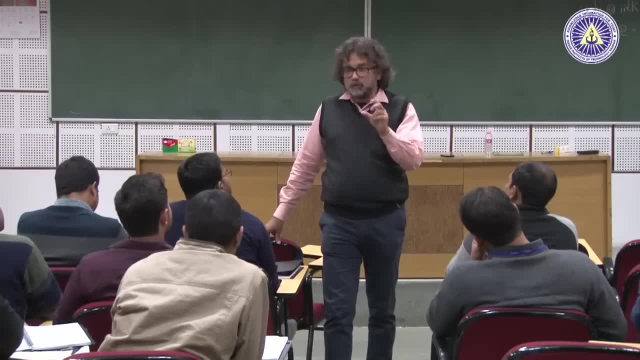 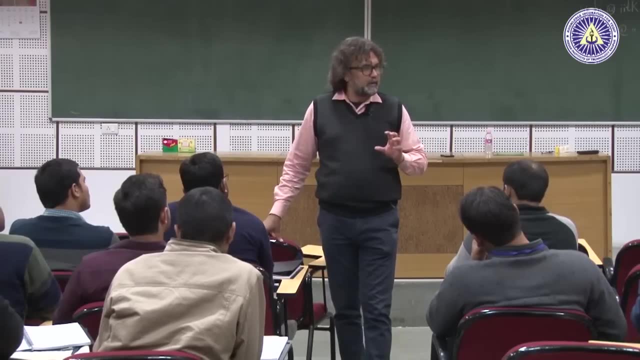 now which one to assume negligible or which one to focus on will depend on the relative magnitude of the things, is it not So? in a human body example, the natural convective heat transfer and radiative heat transfer are almost equal, and your answer has to be: 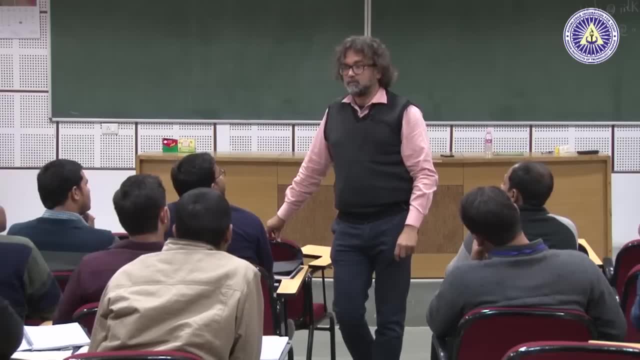 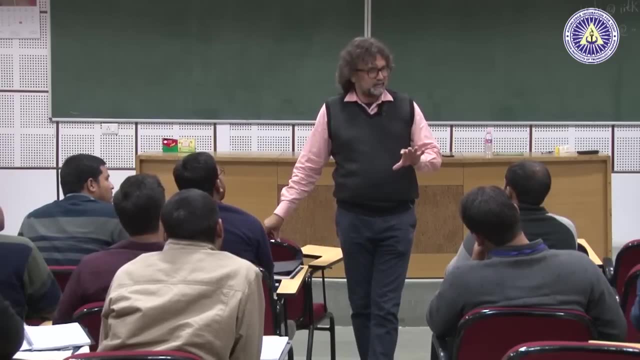 multiplied by 2. yes, you do the calculation, you understand. So this is what I want to stress. you know, in half an hour I cannot tell you everything, but the underlining, let us say, message. the take home message which I want to give is that make an effort. 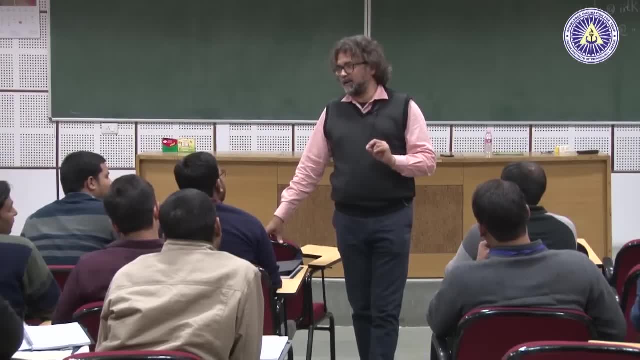 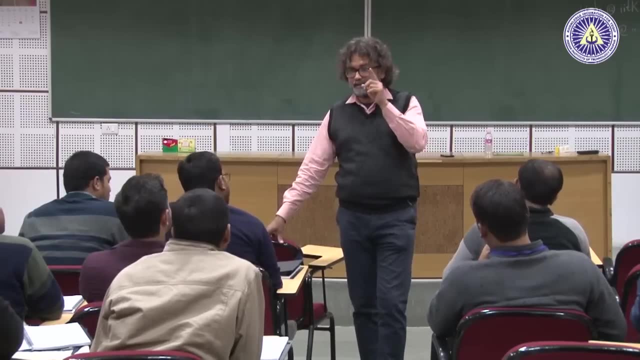 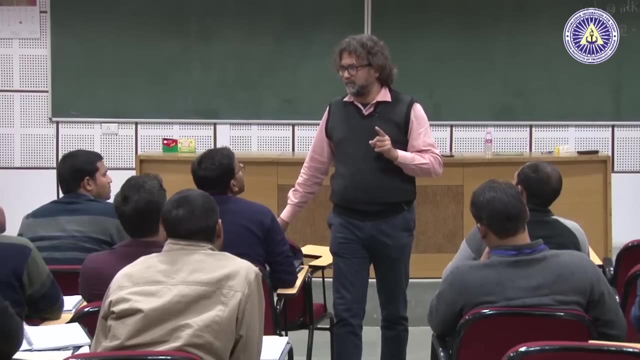 So that the equations which you derive in the class come alive. talk about examples which can be related to that equation. that equation is not a dead equation, otherwise the same equation can be taught by a mathematics student also, a mathematics teacher also, is it not? it is the same differential equation, know, Let us say energy equation, or partial derivate. 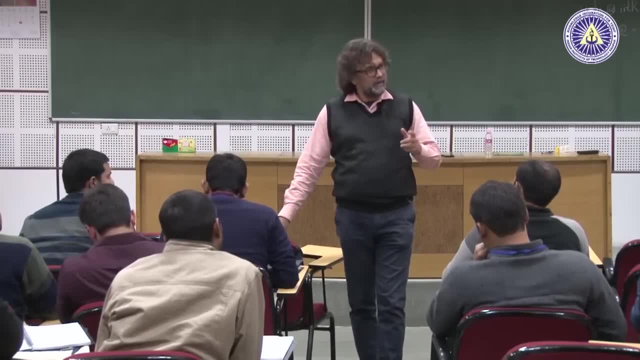 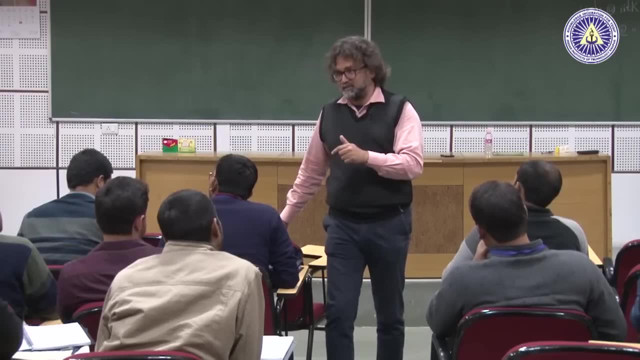 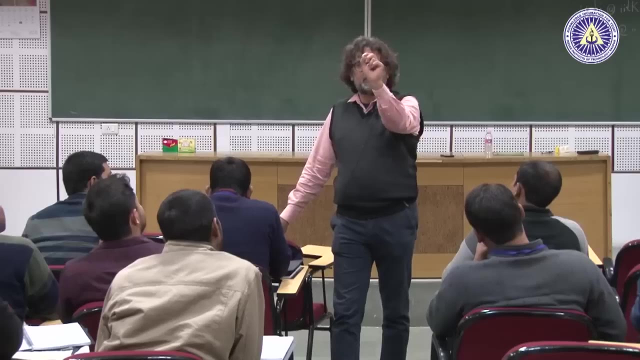 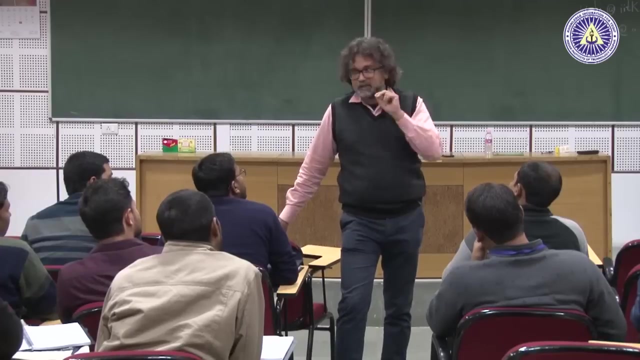 partial equations, which are Navier Stokes equation. it can be taught by a mathematics mathematician also. So why is a mechanical engineering engineer being asked to teach that equation? To derive that equation, boundary condition, Dirichlet boundary condition. you can write it, but do you know what is Dirichlet boundary condition in terms of temperature? how do you? 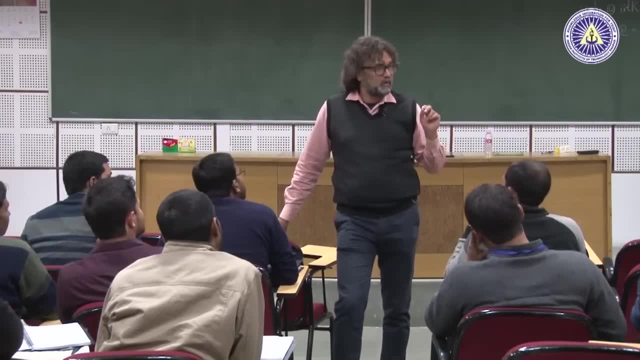 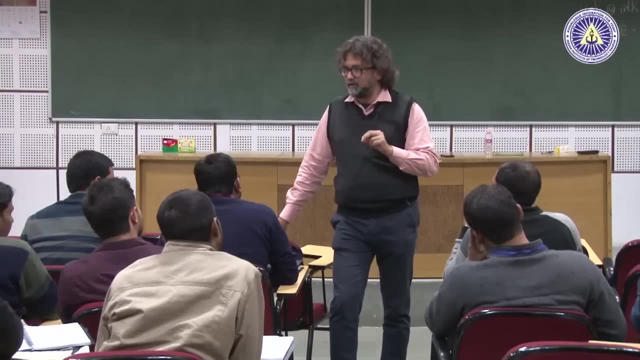 achieve it? which systems are there around you where in insulated boundary condition is really working? or is it really possible to have an insulated boundary condition in real time scenarios? How close can you go to a insulated boundary condition? when you say convective boundary condition, So a system has h is equal to 10, what does it mean? what is that 10? how many systems are? 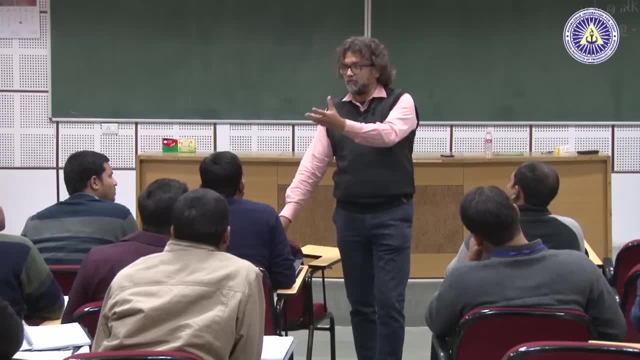 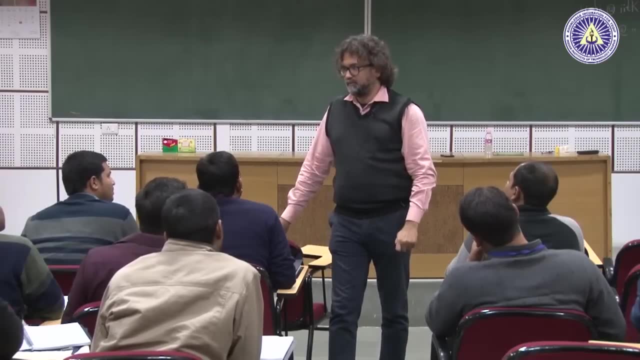 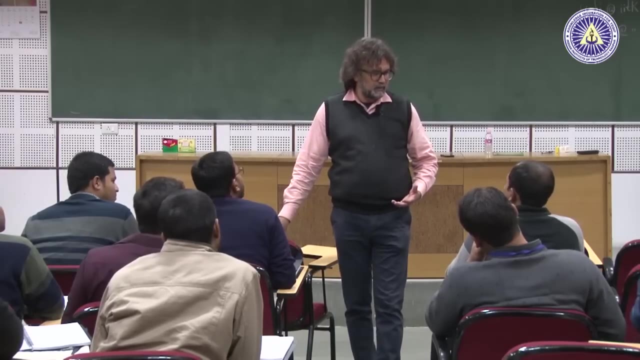 there which have h is equal to 10? how many systems are there? you have a p c, for example. there is a fan at the back, is not it? what is the h in those systems? is it 10? is it 50? is it 200? is it 2000? watts per meter square Kelvin. 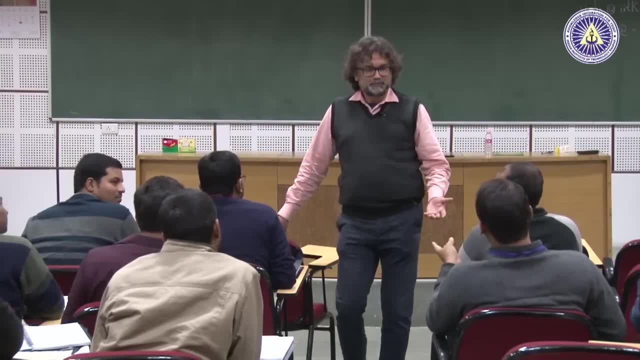 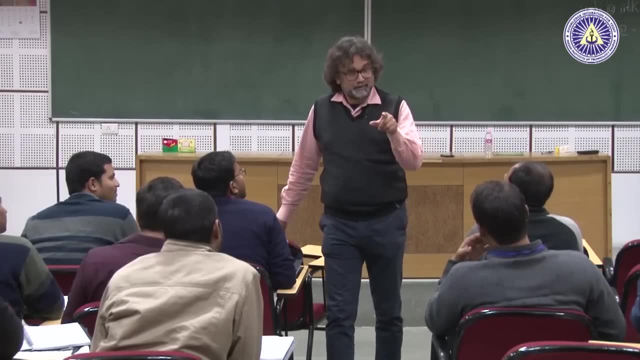 See, there is one order of magnitude coming in this class itself. No, no, there is. it must be around 50. It must be around 50.. It must be around 50.. 50 to 100.. You see, three answers have come. this is important. 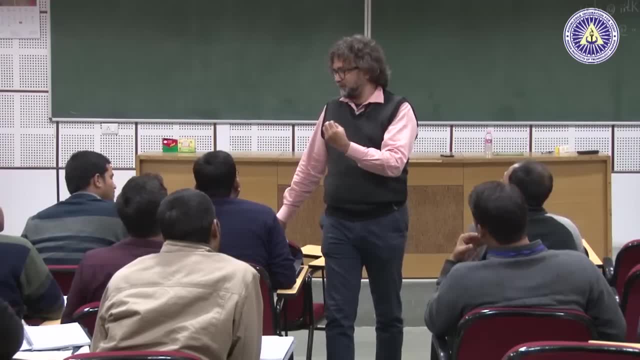 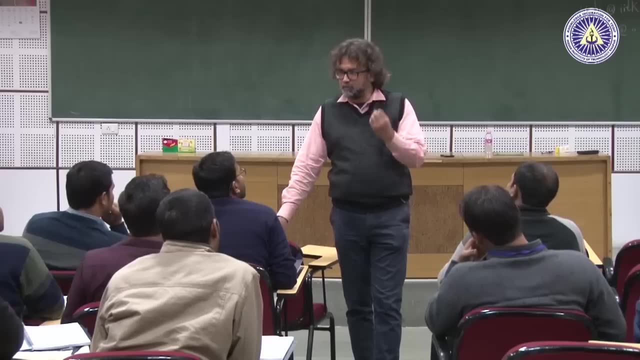 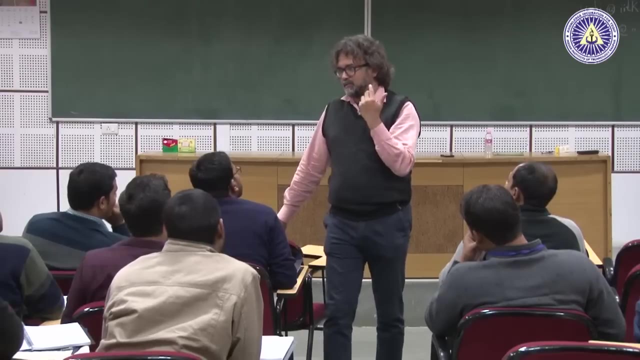 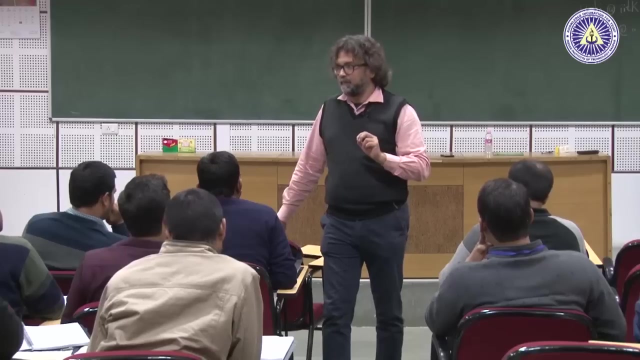 Please try to get real time values and that is why I said some of the books are good. these books have examples, these books have problems wherein the value which has been taken is not just because All these books, the good books, will always assume values Which are very close to real time technological or real time industrial problems. 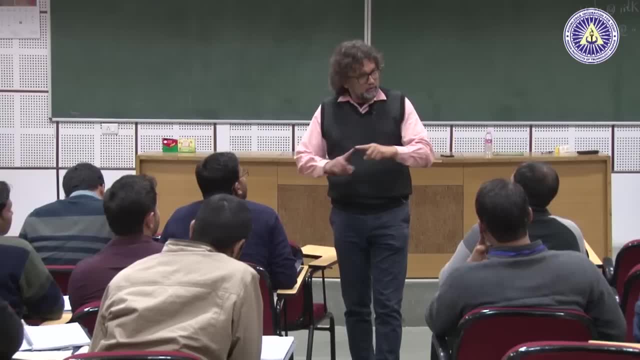 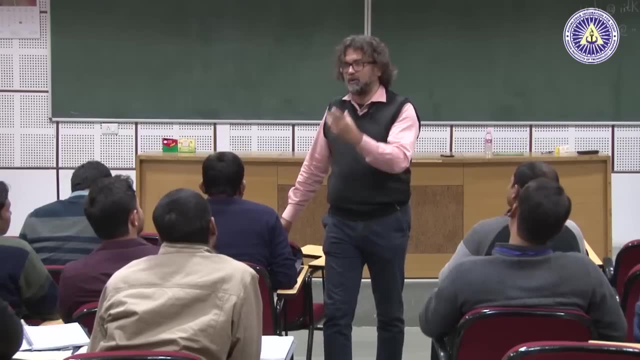 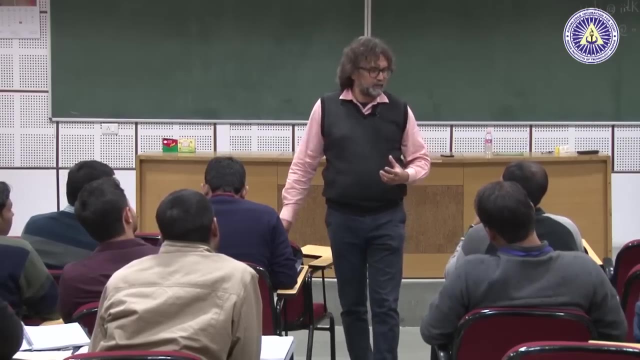 So it is very important for you to get hold of these books, solve these problems, before you go to the class and then get a feeling of what is 100 watt, what is h is equal to 20, which are the systems where h is increasing. what do you mean by low Prandtl number systems? 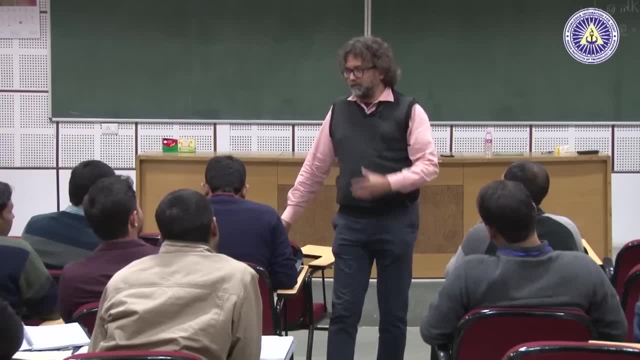 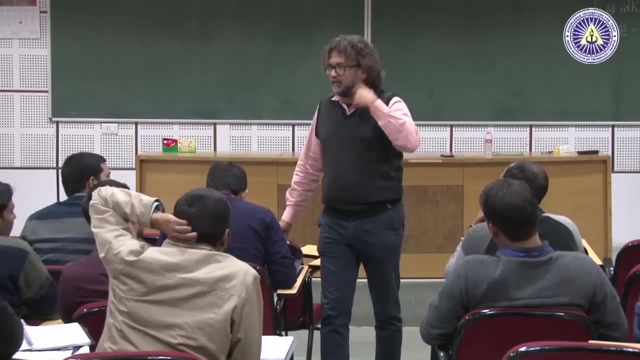 what is the? what is the meaning of high Prandtl number systems? When oil is falling down of a hot wall, is it a low Prandtl number system or a high Prandtl number system? You have to keep thinking about it. if you do that, then your teaching will come alive. 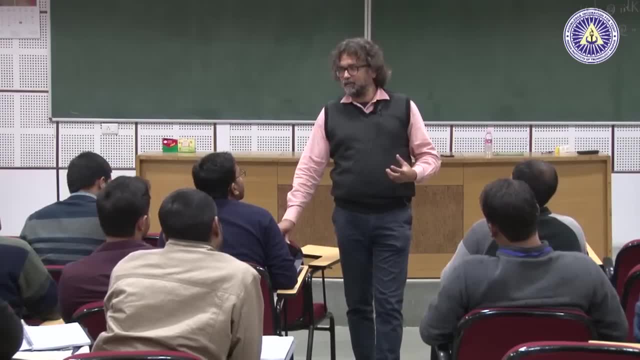 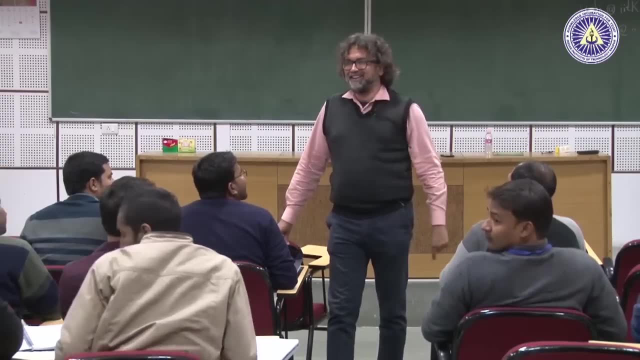 that means people will be happy to come to you, isn't it? and then there is no problem of attendance or anything, is it not? So I think I have run out of my time. no, no, no, that is okay. Malay is already here. 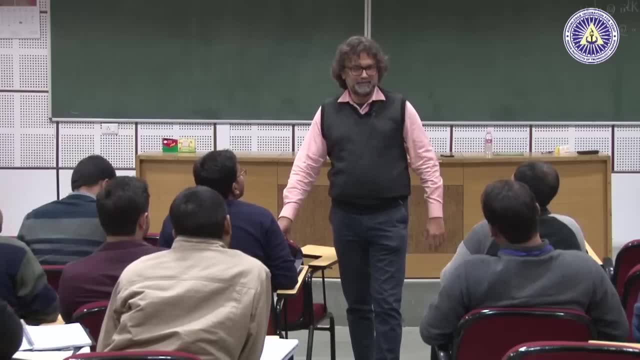 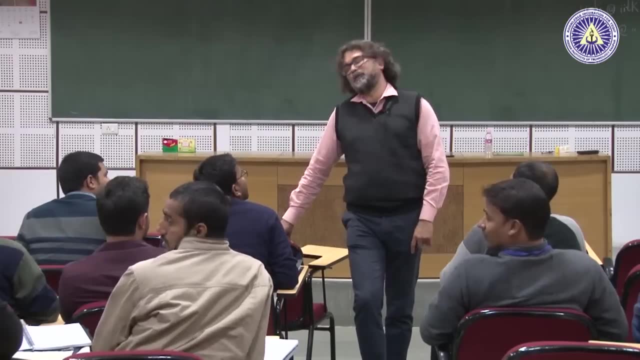 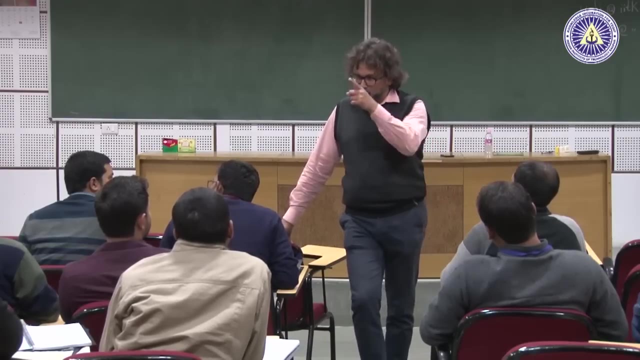 So Malay will also discuss a few things. he is also a fantastic teacher. He has also taught large classes fluid mechanics, not thermodynamics, no, thermodynamics, also fluid mechanics. So he has taught. he has taught large classes, 450-400 students, like 380 students, fluid mechanics. 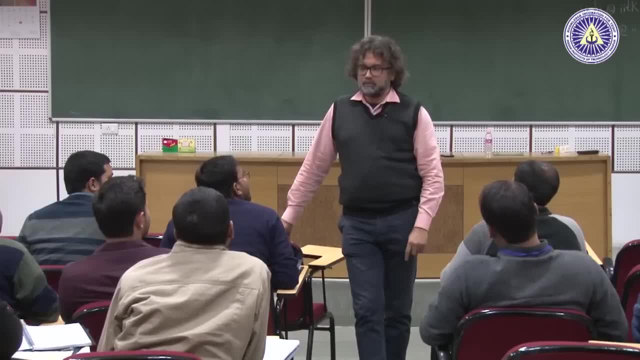 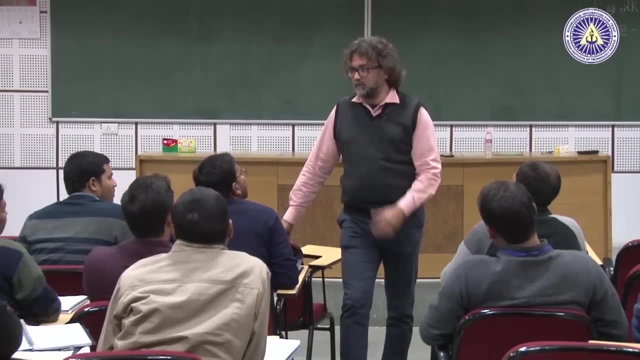 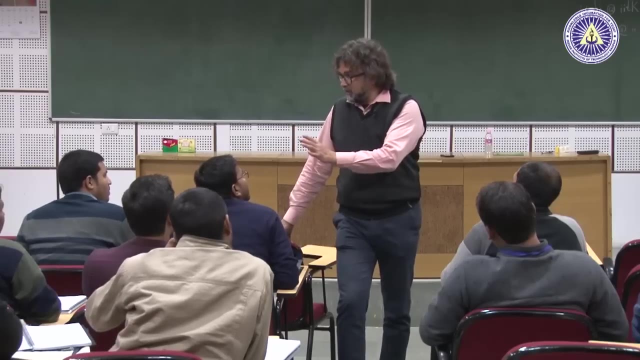 I have taught large classes with thermodynamics. okay, So that also requires enormous amount of you know planning. okay, Malay can be. Malay can give a lot of ideas about how to plan for a class, Because the course is wide, Everything has to be covered and interest also has to be simultaneously, let us say you 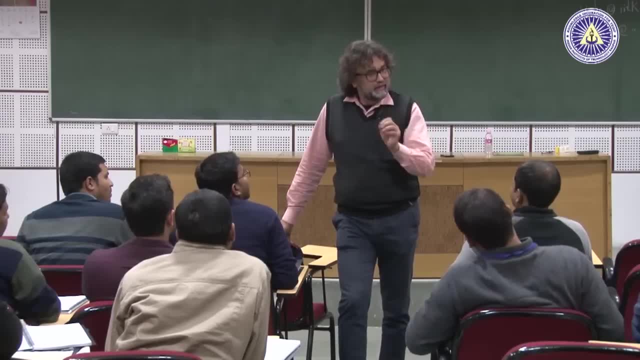 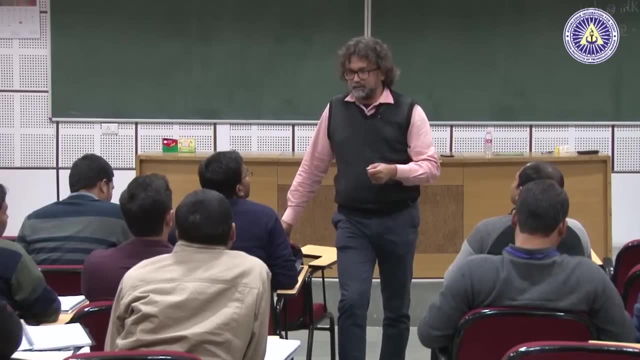 know it has to be kept alive. You cannot leave anything. also, and they are young students, So you have to give them a lot of assignments, you have to make sure that they are doing it. you have to take a quiz also in between, and there are only 40 hours, or even less, 35-36. 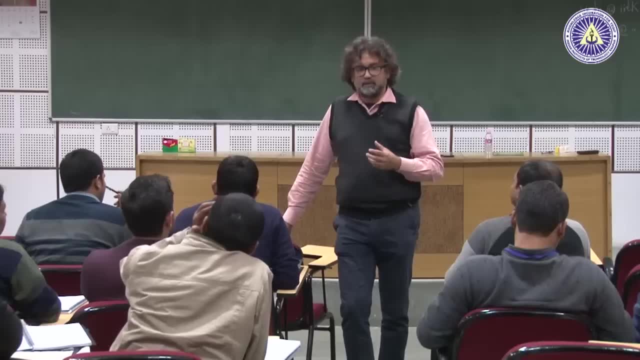 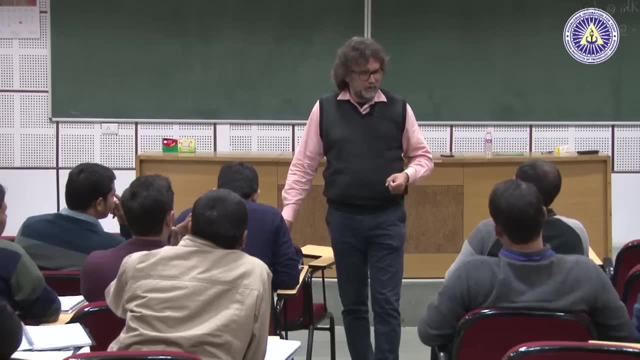 hours which we get in a full semester. So teaching fluid mechanics in 35 hours with lot of time, Lot of interest, lot of examples and derivation and whatever. I have told you how to make it alive and things like that- is very, very challenging job, okay.